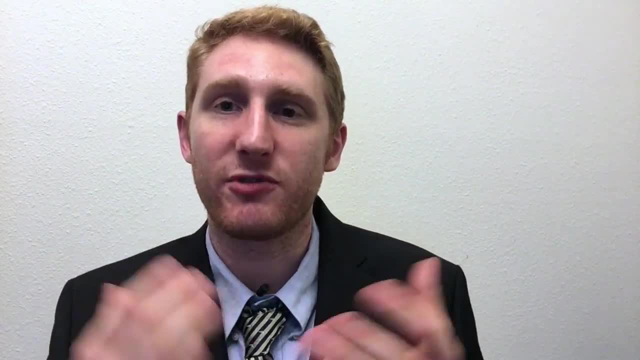 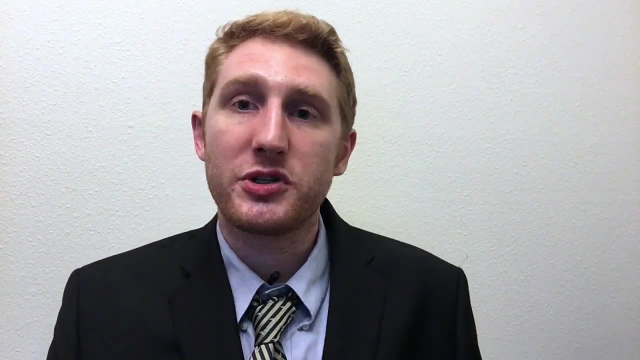 and also in my comment section. so I decided to put together this GED practice test for language arts. Now, if you want help on the essay, I've got other videos on that which I'll link to down below, but you should know this. the essay is only a small portion of your score. Now, this is a little known. 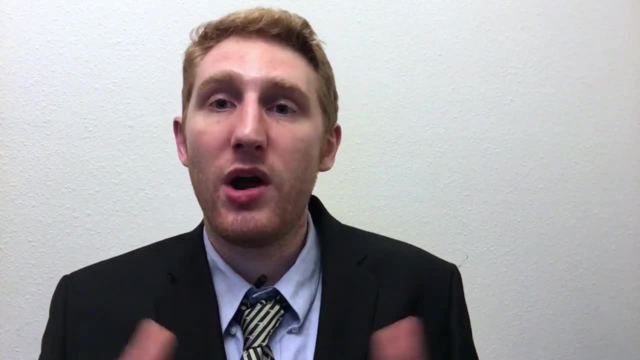 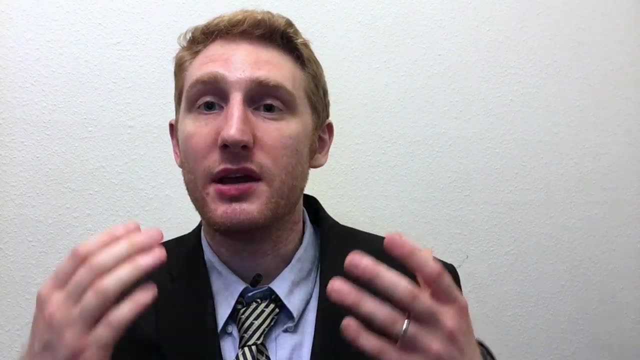 secret. but you can get a zero on the essay and still pass. if you do really well on the multiple choice section, all right. That being said, if you do well on the essay, it's only going to help your score and it can bail you out if you don't do so well on the multiple choice, but the multiple choice is really where you're. 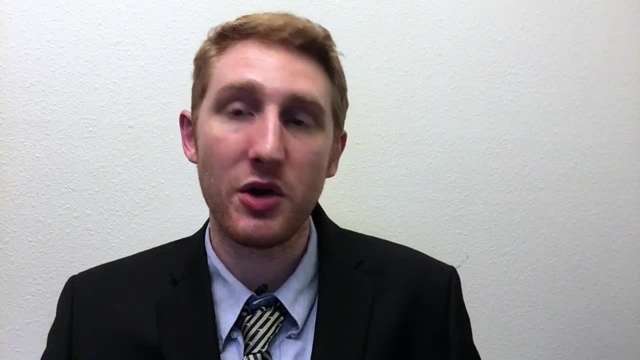 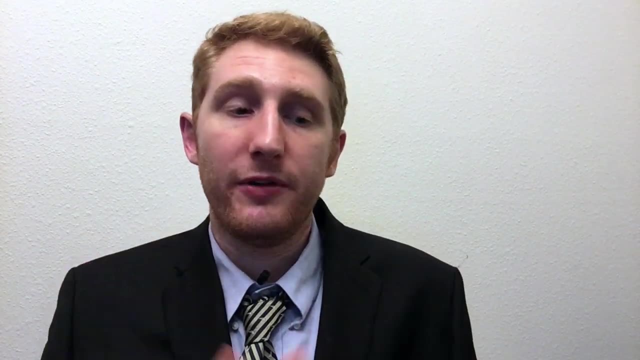 going to earn your money, so to speak, when it comes to the GED language arts section. So in order to help you get the most out of this, I've prepared a printable pdf version down below that you can click on that link down below and you can download that now. Also, I'm going to put in the description: 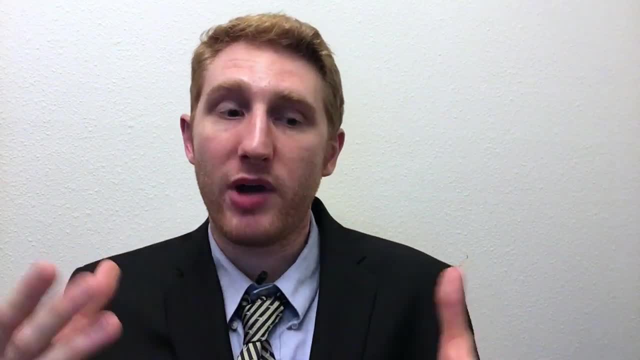 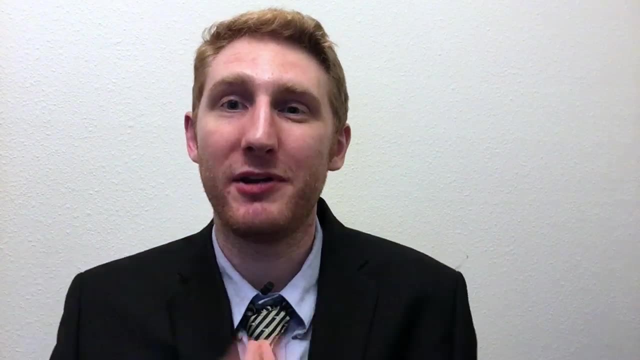 the time that each passage starts and each question starts to skip around, and so that way you can skip back and forth between the passages, hopefully fairly easily, to get the most out of this. So I'm really excited to share this with you guys. Let's jump into it right now. This first excerpt comes from the book The Most Dangerous Game. 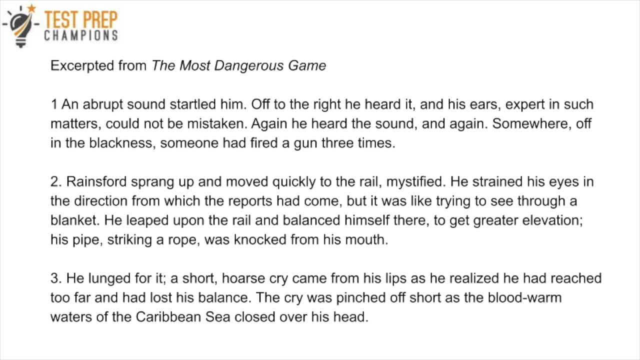 An abrupt sound startled him Off to the right. he heard it and his ears, expert in such matters, could not be mistaken. Again he heard the sound and again, somewhere off in the blackness, someone had fired a gun three times. Rainsford sprang up and moved quickly to the rail, mystified. 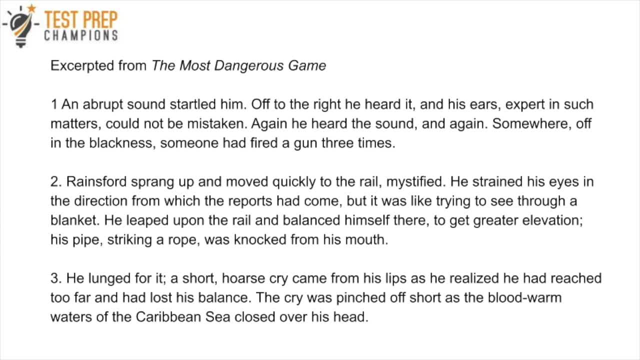 He strained his eyes in the direction from which the reports had come, but it was like trying to see through a blanket. He leaped upon the rail and balanced himself there to get greater elevation, his pipe striking a rope. He then leaped on the rail and balanced himself there to get greater. elevation, His pipe striking a rope. He then leaped on the rail and balanced himself there to get greater elevation, His pipe striking a rope. He then leaped on the rail and balanced himself there to get greater elevation. He then leaped on the rail and balanced himself there to get greater elevation. He. 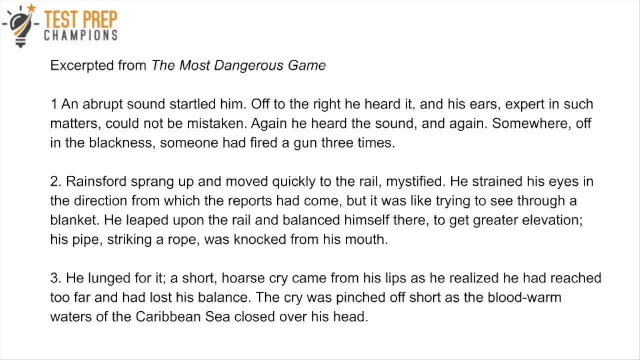 leaped on the rail and balanced himself there to get greater elevation. He lunged forward. A short, hoarse cry came from his lips as he realized he had reached too far and had lost his balance. The cry was pinched off short as the blood-warm waters of the Caribbean. 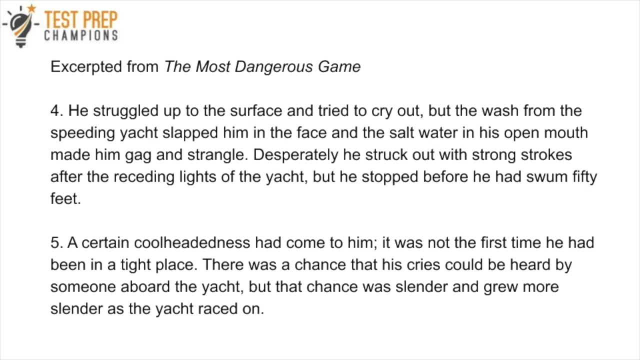 Sea closed over his head. He struggled up to the surface and tried to cry out, but the wash from the speeding yacht slapped him in the face and the salt water in his open mouth made him gag and strangle Desperately. he struck out with strong strokes after the receding lights of the yacht. 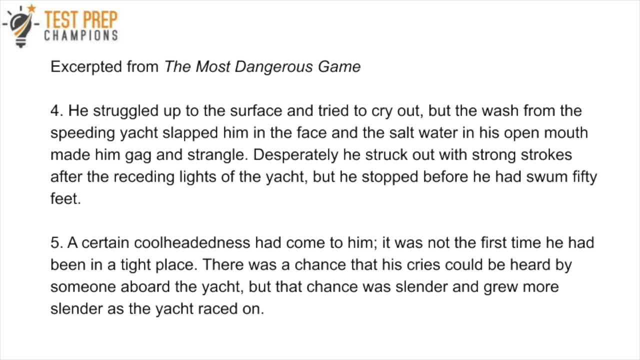 but he stopped before he had swum fifty feet. A certain coolheadedness had come to him. it was not the first time he had been in a tight place. there was a chance that his cries could be heard by someone aboard the yacht, but the chance was slender and grew more slender as the yacht 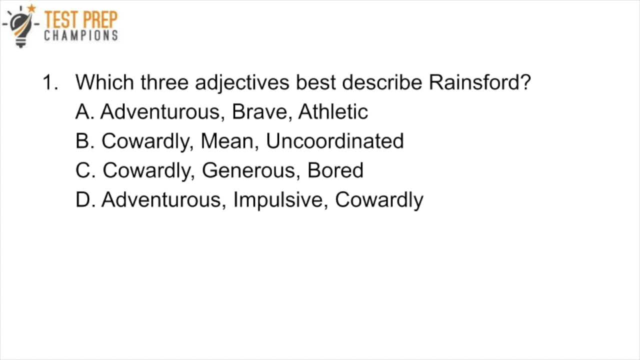 raced on, so question. one reads: which three adjectives best describe rainsford: a- adventurous, brave, athletic. b- cowardly, mean uncoordinated. c- cowardly, generous, bored, or. d- adventurous, impulsive, cowardly. pause the video and try to figure this out. okay, let's go over this. the first: 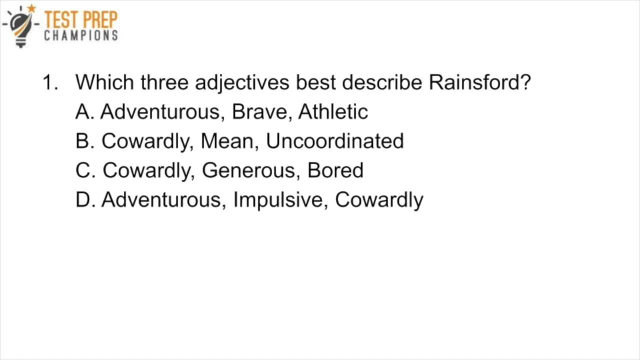 thing you need to know here is what an adjective is. so an adjective is a word used to modify or describe a noun or pronoun. a noun is a person, place, thing or idea, and a pronoun takes the place of the noun. it substitutes for the noun. so an adjective is used by an author for a description. 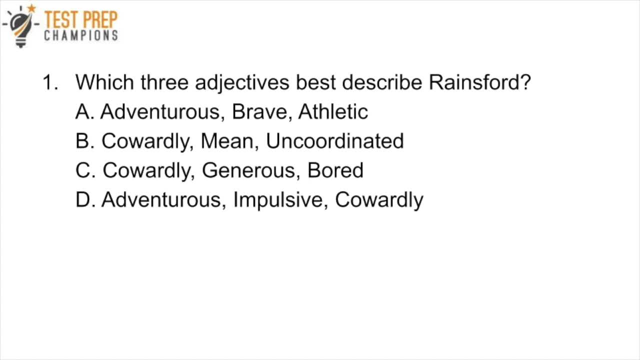 to tell us about a character or give a description here. so what we want to do here is refer to the passage and try to figure out which adjectives best describe rainsford. so, and the answer is going to be a. so we get evidence that he's brave and adventurous from paragraphs one and five, where 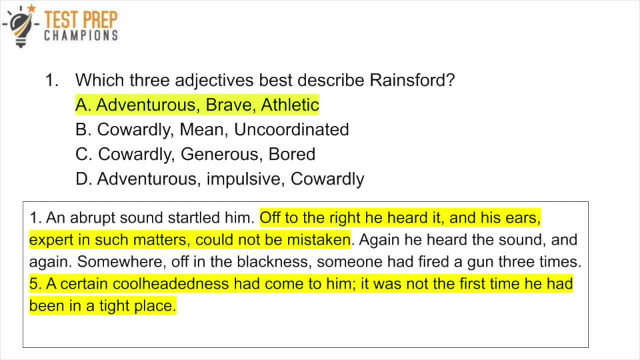 it says that off to the right. he heard it in his ears. expert in such matters could not be mistaken. so this is suggesting to us that he's heard gunshots multiple times. and we also have to look at paragraph five, where it says a certain cool headedness had come to him. it was not the first time he had been in a tight place. so 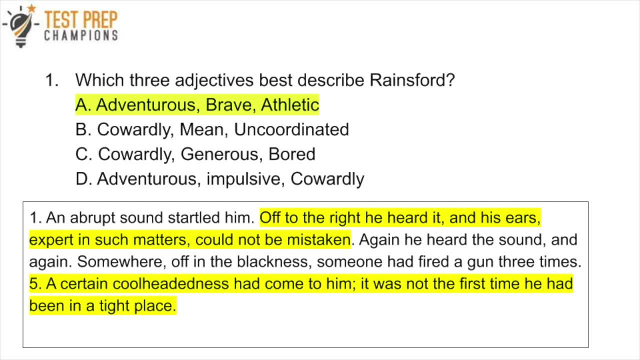 cool headedness means that he's calm or collected. he's cool under pressure. he's keeping a cool head under pressure, and this isn't the first time that he's been in a tight place like this. so we can take these two pieces of evidence and we can conclude that he's adventurous and brave. 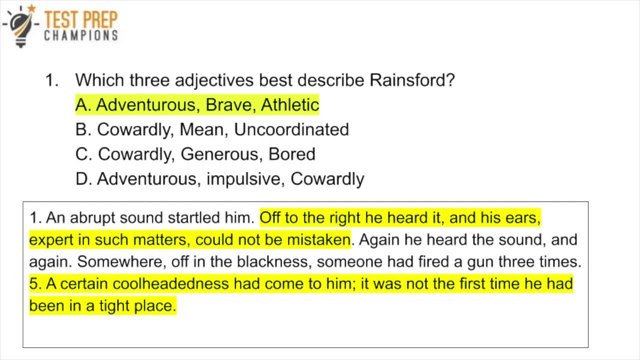 okay, so he's not cowardly, right, because if he was cowardly then he wouldn't be cool under pressure, he wouldn't have cool headedness, all right, and so also, what about? mean? well, it's not telling us anything about his character, right? so there's no interactions with other characters going on here. there's a yacht, but we don't know. 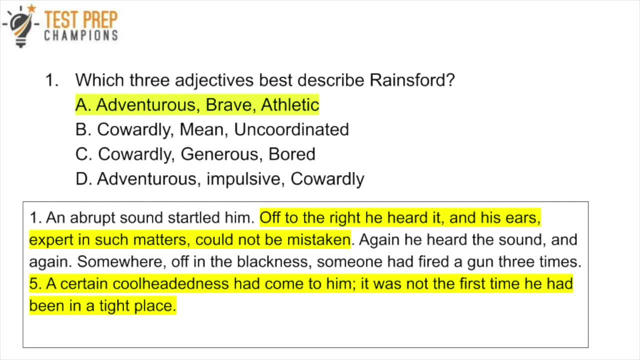 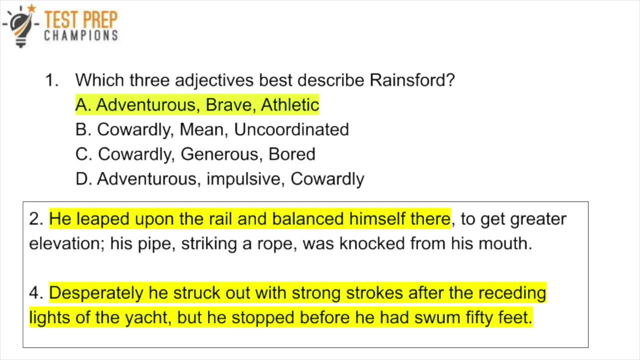 anything about his interaction with the driver on the yacht. so we can't say that he is mean and we can't say that he's generous. so neither of those are going to help us out. but what about athletics? so we want to look at paragraphs two and four, where it says he leaped upon the rail and balanced. 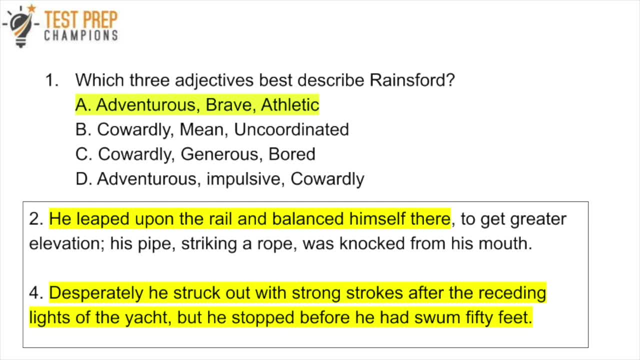 himself there, one sign that he's athletic. and four where it says desperately struck out with strong strokes after the receding lights of the yacht. but he stopped before he swung 50 feet, so he's striking out with strong strokes here. so that's another indication that he may be athletic, all right. 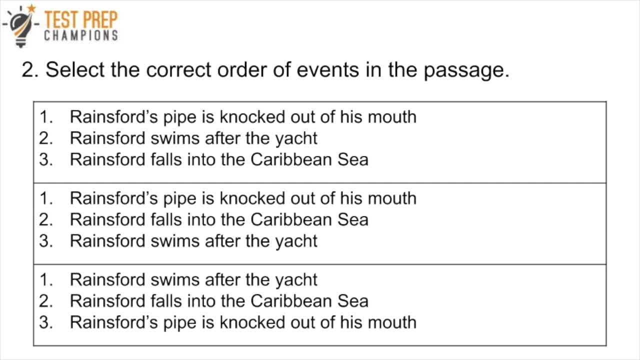 okay. so question two says to select the correct order of events in the passage, and on screen you're shown three different boxes. so pick the box that shows the correct order of events in the passage. pause the video and try to do that now. okay, let's go over this. so the second box, of course. 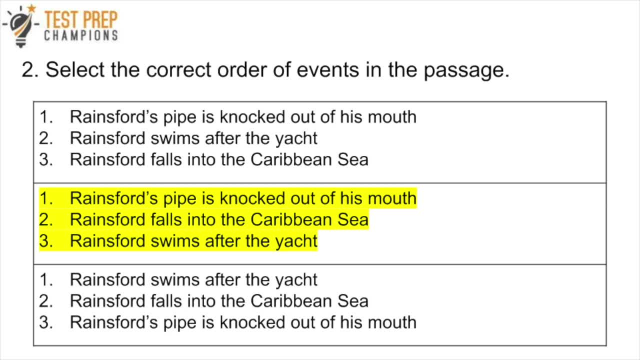 is the correct order here. second box shows the correct order and to get this one right you just have to remember the sequence of events in the story, or look back at the story and then pick the events in the right order. so remember rainsford first heard gunshots, then he jumps onto the rail. 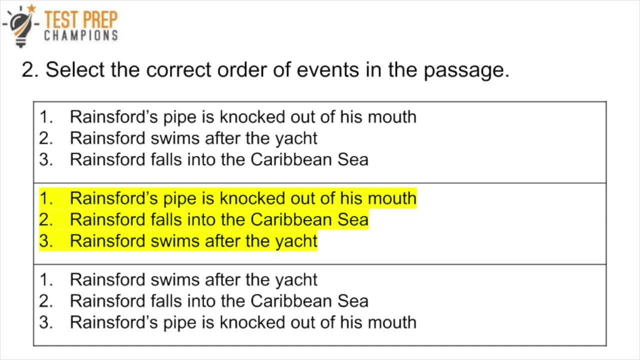 and then, once he jumped onto the rail, he tried to look in the direction of the shots and his pipe struck the rope and the pipe was knocked out of his mouth. then he tried to catch his pipe but lost his balance and he fell into the sea. then, once he fell into the sea, he tried to swim. 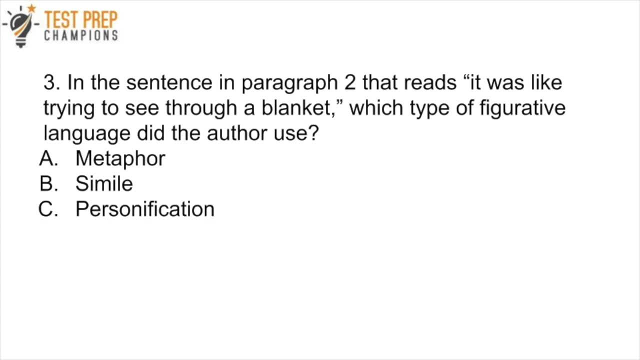 toward the yacht, so that's why the second box is correct. okay, question three, and the sentence in paragraph two that reads: quote: it was like trying to see through a blanket quote. which type of figurative language did the author use? a metaphor, b, simile or c personification? 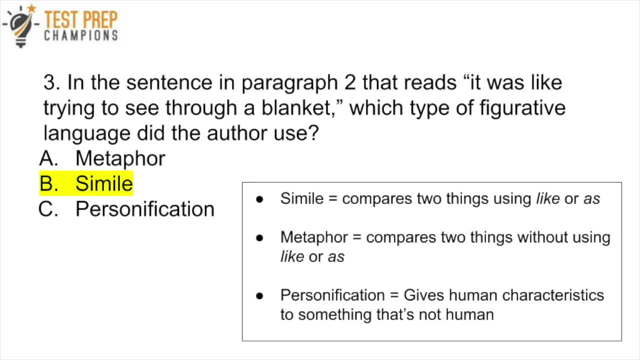 pause the video and try to figure this out. okay, let's go over these. so these are three types of figurative language that you're definitely going to want to know about, and the correct answer is be similarly so. similes compare two things using the words like or as so when the author says it. 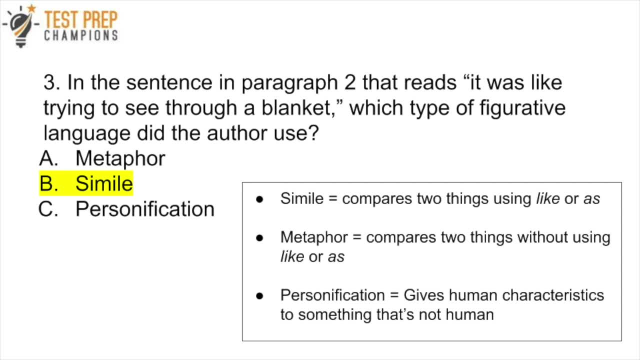 was like trying to see through a blanket. the word like is our key: that this is a simile. so metaphors compare two things. but metaphors don't use the words like or as and persona, and in personification the writer gives human characteristics to something that's not human. so, for example, during: 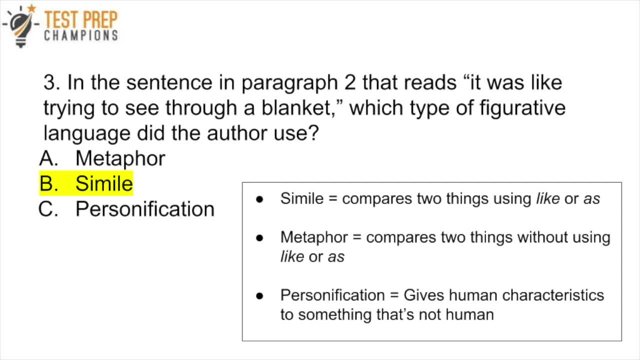 a storm. if the wind blows really hard, it might kind of sound like someone's knocking on the door, and so the author might say something like the wind knocked on the door, which would be giving human characteristics to something that's not human, which is personification. so question four. 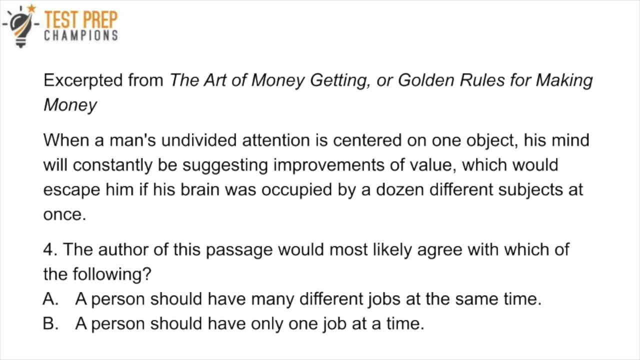 is paired with an excerpt here that reads: when a man's undivided attention is centered on one object, his mind will constantly be suggesting improvements of value. then question four reads: the author of this passage would most likely agree with which of the following: a- a person should have many different jobs at the same time, or b- a person should have 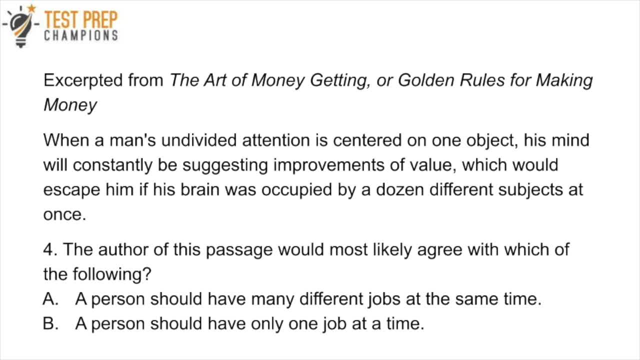 only one job at a time. pause the video and try to figure this out. the answer here is b. the author would most likely agree that a person should have only one job at a time, and to get this question right we have to make an inference here. an inference is a guess you make based on the given. 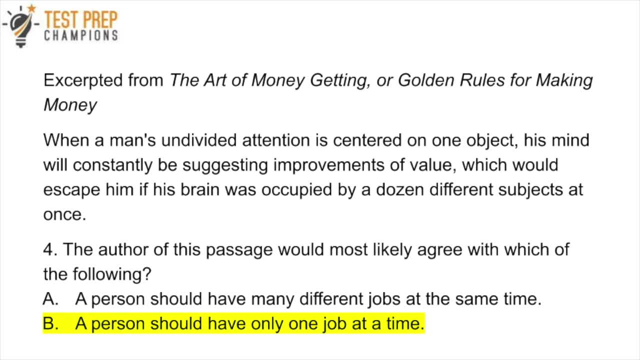 information and also your own knowledge and experience. so if you have the answer a- b and you're not sure what to do with the answer a- b and you're not sure what to do with the answer b in real life, So to make an inference successfully you have to read and ask: what does the given 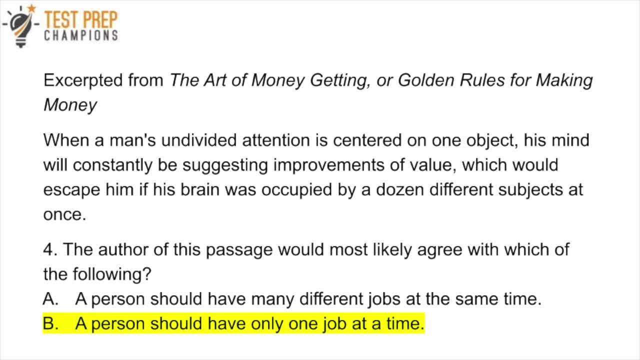 information point to. And so since he's talking about a man's undivided attention being better than having his mind on multiple things at once, we can agree here that he would most likely agree that a person should only have one job at a time. So question five says: choose the phrase that best. 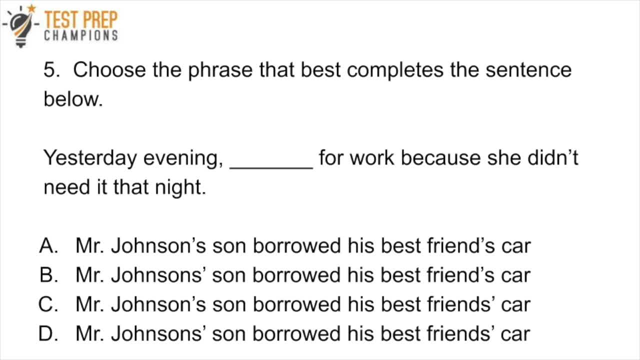 completes the sentence below: Yesterday evening blank for work, because she didn't need it that night. And then the blank should go: Mr Johnson's son borrowed his best friend's car. So what's the correct way to write? Mr Johnson's son borrowed his best friend's car. That's what you want to. 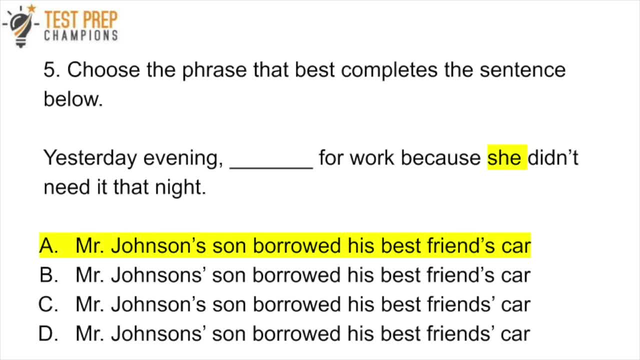 find here. So buzz the video and try to do that now. Answer A is the correct answer here, And the question is really testing your knowledge of apostrophes. So there are two general rules that you need to know about apostrophes. So if we're talking about a person, object, place or idea, 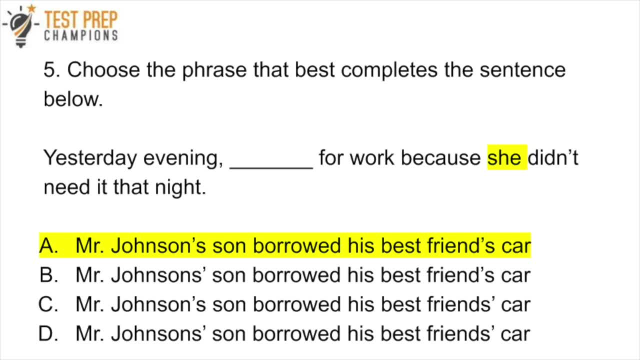 that belongs to one person, you add an apostrophe followed by the letter S. Now if the person, object, place or idea belongs to multiple people, then you put an S first and then an apostrophe. So these are just two general rules of thumb here. So when we're talking about Mr 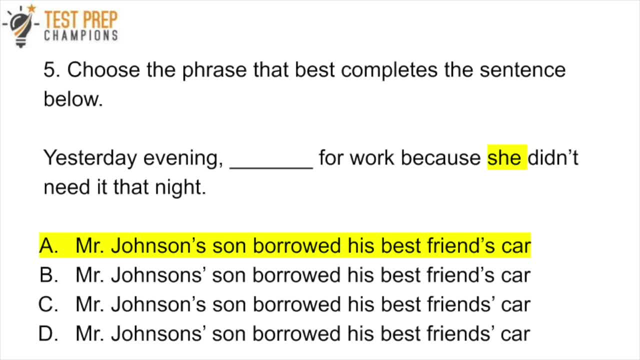 Johnson, who is one person. we put the apostrophe first, then the letter S. Now, looking at the word friend, we have to read really carefully in the excerpt to see where it says she didn't need it that night. So the word she here tells us that we're reading about just one person. So it's not. 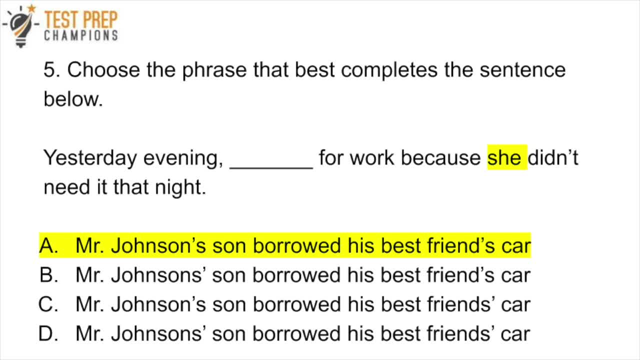 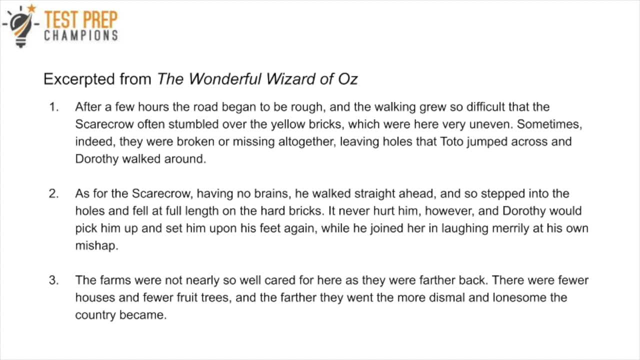 a group of best friends, So it's just one person's car. So we add an apostrophe after friend, followed by an S, And that's why A is the correct answer. Okay, the next set of questions come from a new excerpt here, And this is from the book The Wonderful Wizard of Oz. So if you've seen the 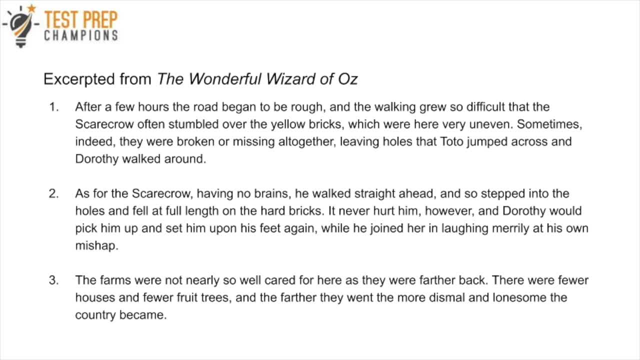 book. you know that you haven't, And I'm going to read through this excerpt kind of fast. but you can pause the video and refer to this. Take your time reading it. So after a few hours the road began to be rough and the walking grew so difficult that the scarecrow often stumbled over. 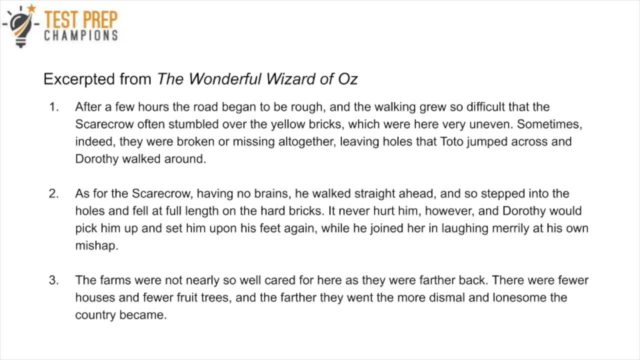 the yellow bricks, which were here very uneven. Sometimes, indeed, they were broken or were missing altogether, leaving holes that Toto jumped across and Dorothy walked around. As for the scarecrow, having no brains, he walked straight ahead and so stepped into the holes and fell at. 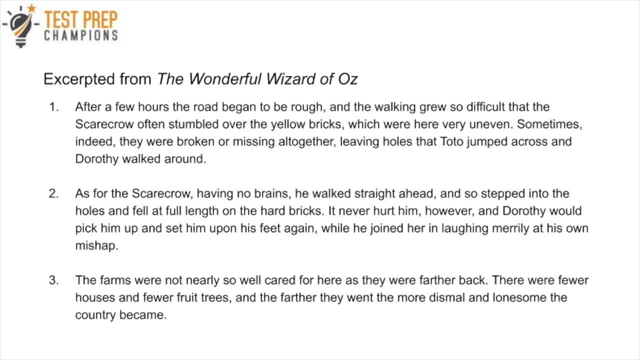 full length on the hard bricks. It never hurt him, however, and Dorothy would pick him up and set him upon his feet again, while he joined her in laughing merrily at his own mishap. The farms were not nearly as well cared for as they were farther back. There were fewer houses and fewer 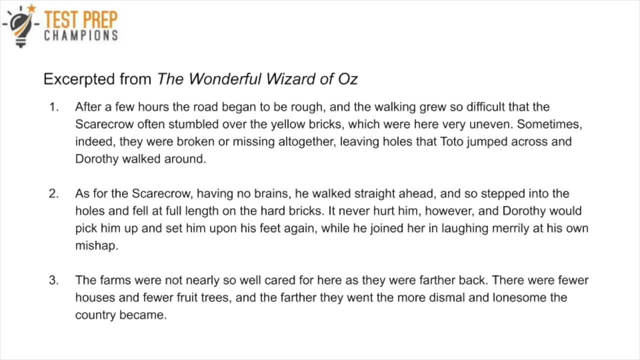 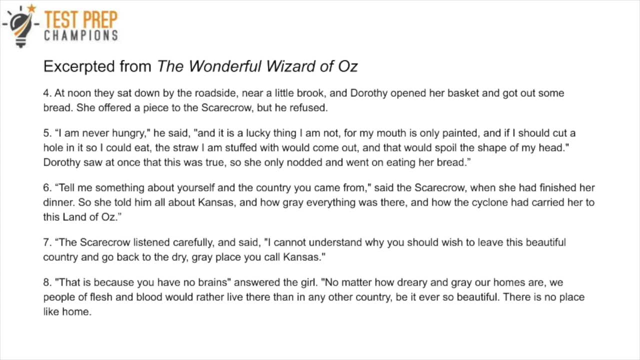 fruit trees, and the farther they went, the more dismal and lonesome the country became. At noon they sat down beside the roadside near a little brook and Dorothy opened her basket and got out some bread. She offered a piece to the scarecrow, but he refused. I am never hungry, he said, and 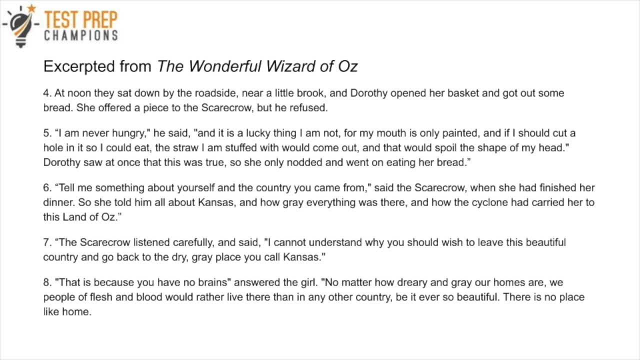 it is a lucky thing I am not, for my mouth is only painted, and if I should cut a hole in it so I could eat the straw, I am stuffed with what comes next. I am not hungry, he said, and I am not. 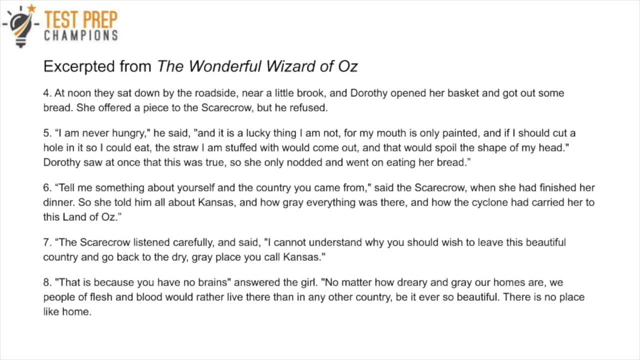 out and that would spoil the shape of my head. Dorothy saw at once that this was true, so she only nodded and went on eating her bread. Tell me something about yourself and the country you came from, said the scarecrow when she had finished her dinner. So she told him all about Kansas. 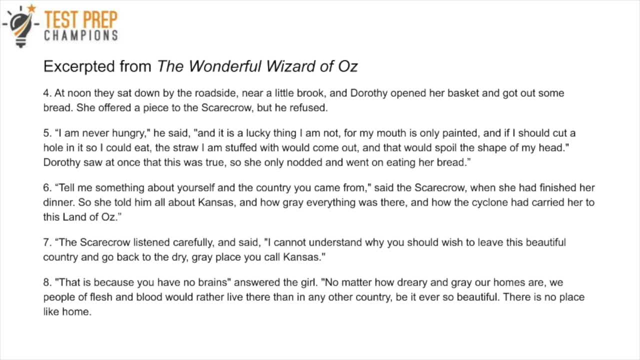 and how gray everything was there and how the cyclone had carried her to this land of Oz. The scarecrow listened carefully and said: I cannot understand why you should wish to leave this beautiful country and go back to the dry, gray place you call Kansas. That is because you. 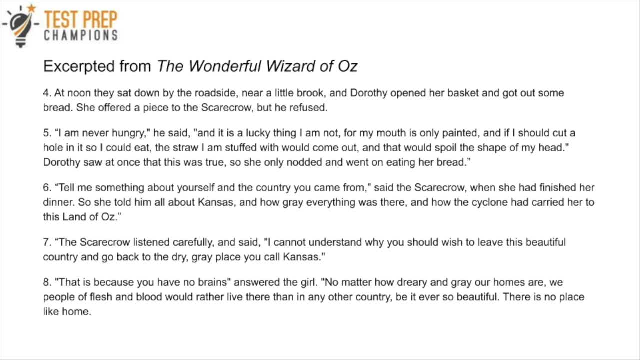 have no brains, answered the girl. No matter how dreary and gray our homes are, we people of flesh and blood would rather not be there. I am not hungry, he said- and it is a lucky thing I am not there than in any other country, be it ever so beautiful, There is no place like home. 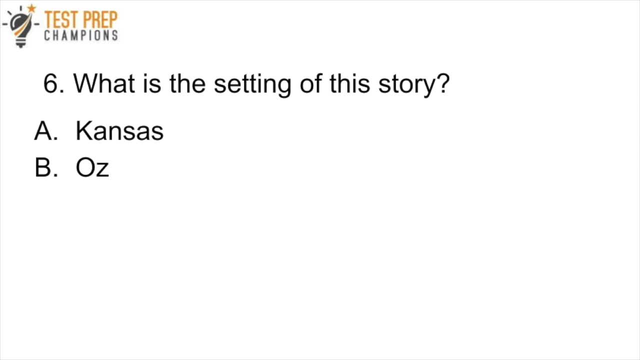 Okay, time for the next question. What is the setting of the story? A Kansas or B Oz? All right, go ahead, pause the video and try to go over this. Try to do this one, then we'll go over it. Okay, let's go over how to do it. So, basically, if you like, I said earlier, 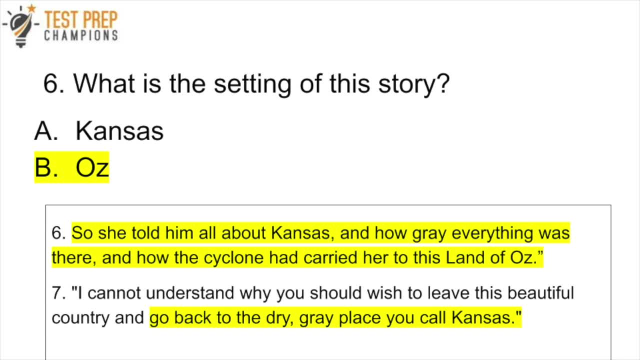 if you know the story of The Wizard of Oz, just pretend that you don't and make sure that you can use the context clues to get the answer here. So, first of all, what is the setting? Well, the setting of a story is just a setting of a story. So if you know the story of The Wizard, 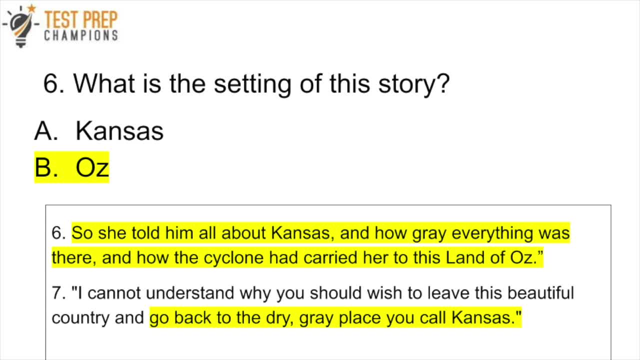 of Oz, just where the story takes place. So it's either in Kansas or it's in Oz. And so in the passage we have to look at paragraph six, where it says so: she told him all about Kansas and how gray everything was there and how the cyclone had carried her to this land of Oz. So 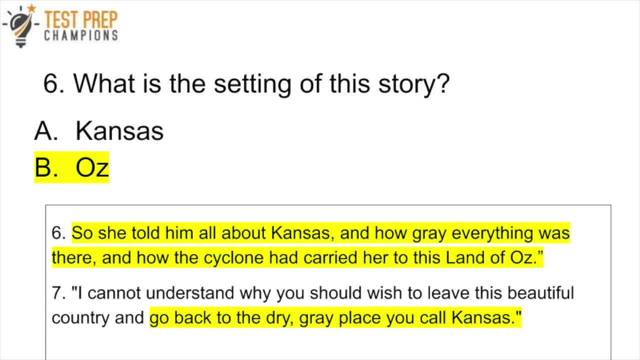 we have to look at two words here. So the word so it's telling us that she started in Kansas, right, And the cyclone carried her to this land of Oz. The word this implies and tells us that she's now in Oz. Also, look into paragraph seven, okay, where the scarecrow is talking about leaving. 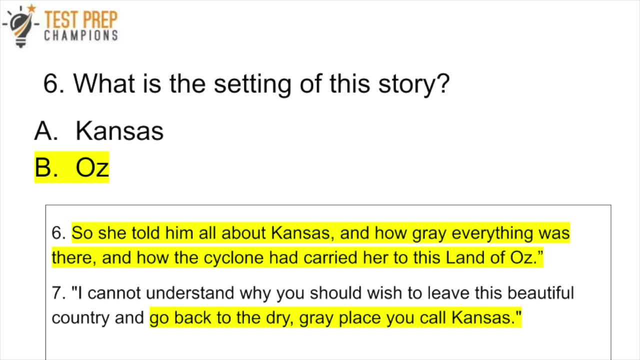 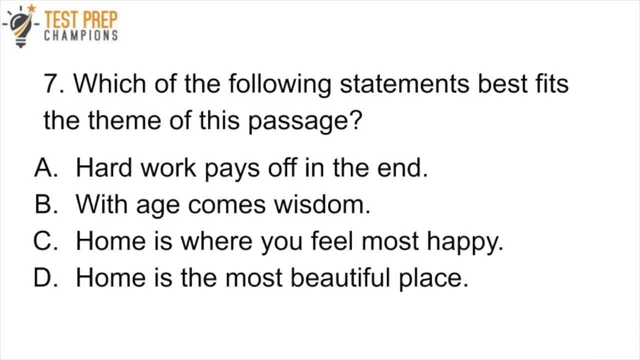 to go back to Kansas. So if she wants to go back to Kansas, all right, then logically she's not in Kansas now she's in Oz. Question seven reads which of the following statements best fits the theme of the passage: A- hard work pays off in the end. B- with age comes wisdom. C- home is where. 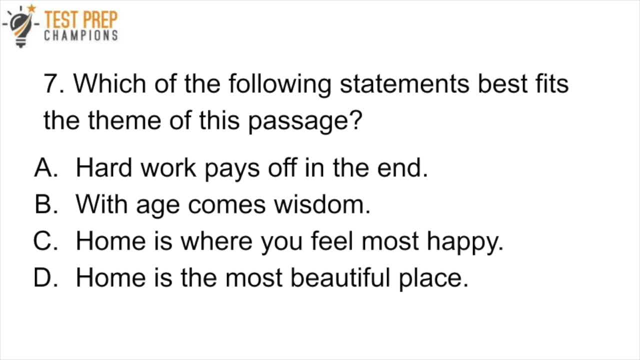 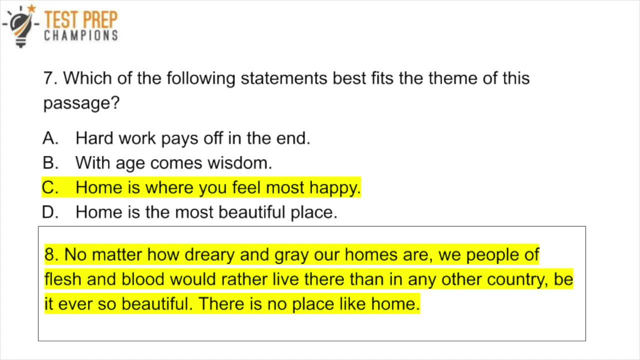 you feel most happy, Or D- home is the most beautiful place. Go ahead and pause the video. So question seven. the answer is C- home is where you feel most happy. So the first thing you have to understand here is: what does the word theme mean? Well, the theme is just the message that 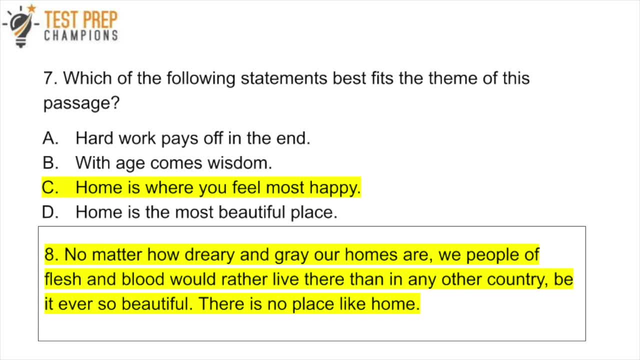 the writer wants to communicate to the reader. The theme is usually a very general statement that the author wants to make about the human experience or about life in general. So the theme might be directly stated by the author, but in many cases the theme is not stated by the author. 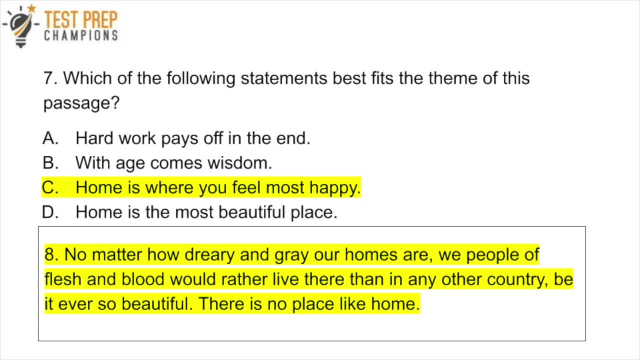 and you're going to have to infer it from what's going on in the story. So, to figure out the theme, some places that you can look are: what's going on with the characters, What are the characters in the story? So you can also ask yourself the question: what is the writer trying to tell us? 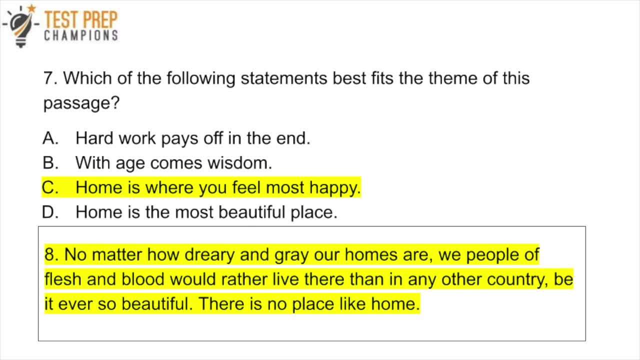 here. What message is the writer trying to communicate to us about life in general? All right, And so what we can do here is use process of elimination to roll out A and B. And the reasons are because hard work and that has nothing to do with the passage. So there was nothing about hard. 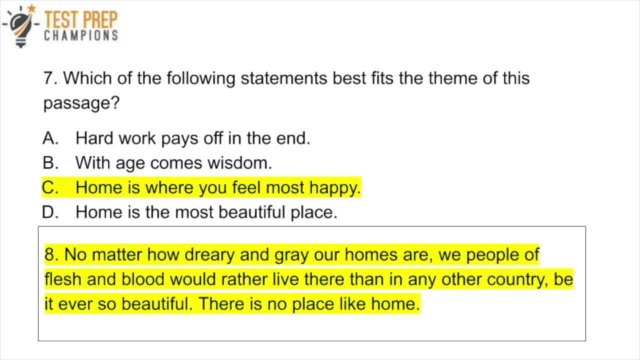 work discussed in the passage Same with: with age comes wisdom. All right, So is the author really trying to communicate the message to us about hard work paying off or about becoming more wise as you age? Well, none of these themes. like I said, these aren't themes that even came up in. 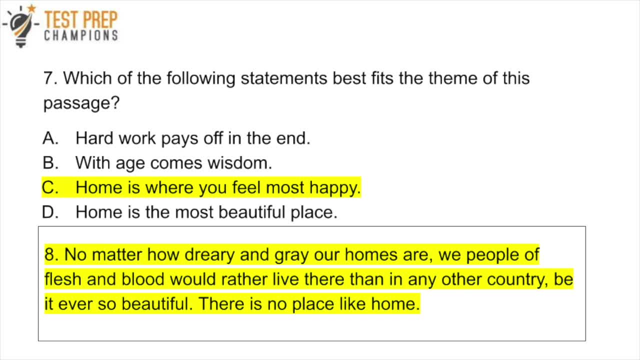 the passage. These aren't even mentioned, So roll those out Now. through process of elimination, we are left with C and D. So C reads home is where you feel most happy and D reads home is the most beautiful place. So here's a general tip for multiple choice tests. So whenever you get two, 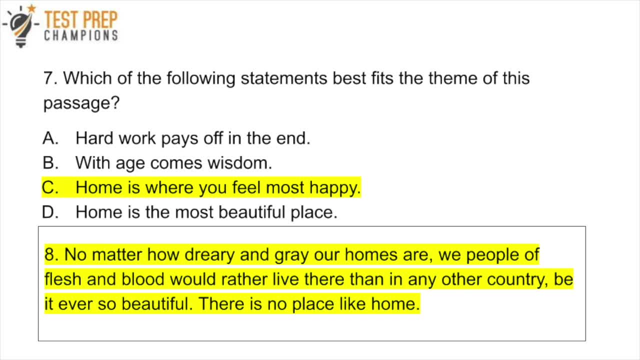 answers that contradict each other and can't both be right. there's a good chance that one of them is the correct answer. Now, this doesn't always work, but more often than not the trick will work. So right away we draw our attention to C and D. Home is where you feel most happy. 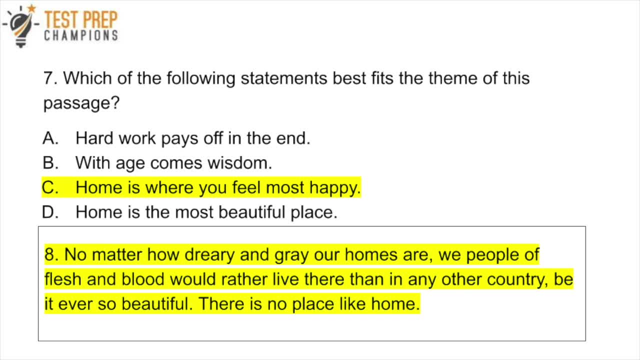 Your home is the most beautiful place, So they can't both be right here. So one of these is correct and it happens to be C. And we see the evidence for C from passage eight, where it says: no matter how dreary and gray our homes are, we people of flesh and blood would rather live there. 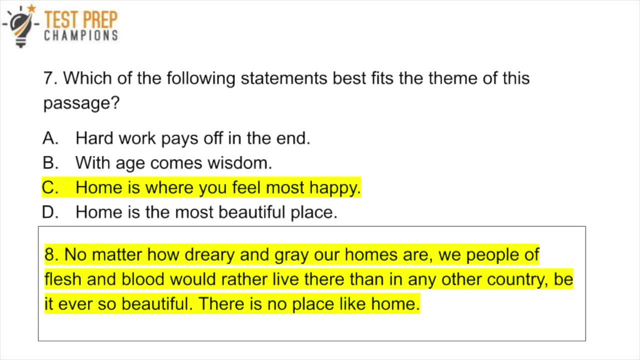 than in any other country, be it ever so beautiful, There is no place like home. So what Dorothy is saying here is that, even though Oz might be more beautiful than our home, even if it's ever so beautiful, she doesn't care. There's no place like home. And so that's the evidence for C. 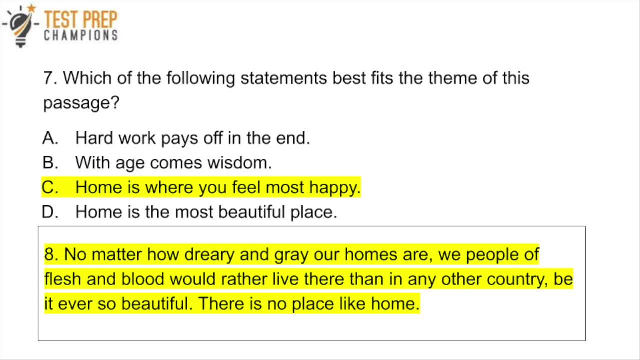 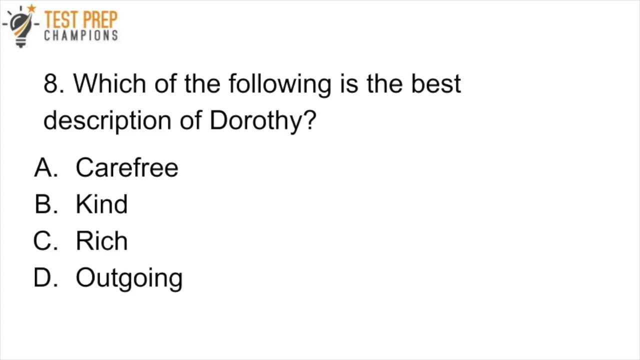 That's why we can conclude that the theme of this excerpt is: home is where you feel most happy. So the answer here is B kind. So why is this the right answer? Well, first of all, for A, we don't see evidence that she's carefree. In fact, we see the opposite. Remember. 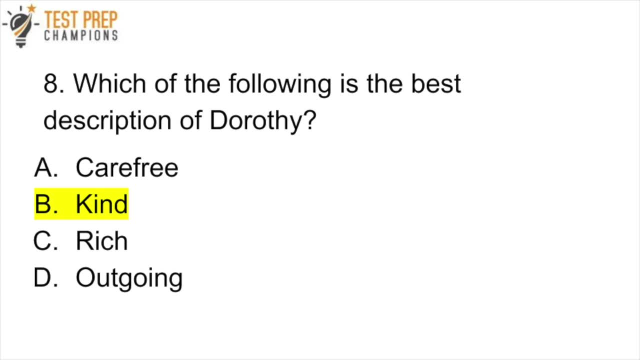 she cares a lot about going home here, and she also seems to be very caring for the scarecrow here. All right, And so let's skip ahead. Let's skip talking about B, Let's go to C here. So their financial status is never mentioned, So we don't know anything about. 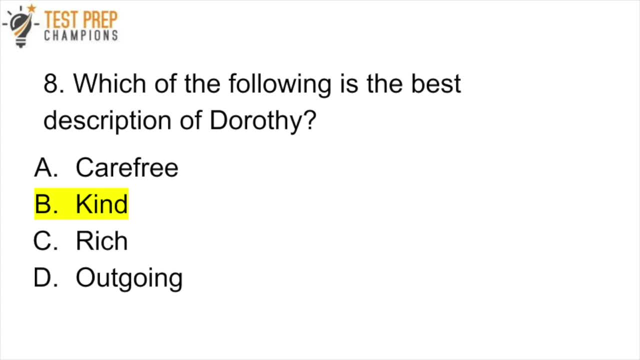 whether or not she's rich. So, as far as D outgoing, well, why is D not the right answer here? Well, first of all, what does it mean to be outgoing? Well, being outgoing means that you like to talk to people a lot, right? So she may in fact be outgoing, or she might be not. We don't really. 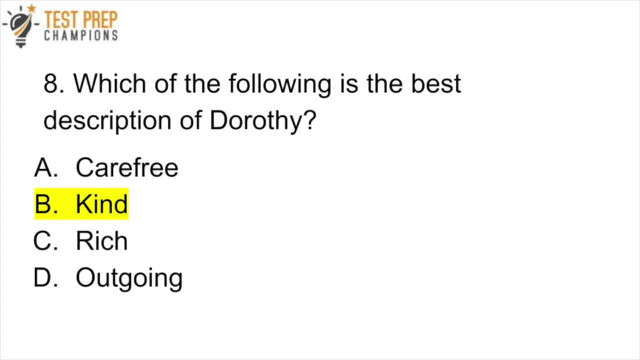 know, though, right, The only character in the story that she talks to is the scarecrow, So she's talking to one person. So we don't know if she's outgoing or not, So we don't know if she's not. So she may be, but we can't confirm it, And we also can't disconfirm it. So remember that. 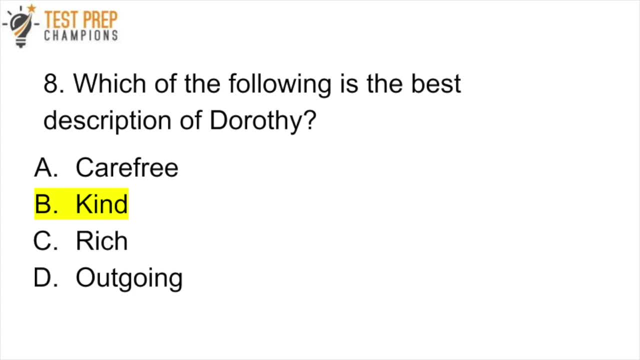 word best in the question. it says which of the following is the best description of Dorothy? So even though we can't confirm or disconfirm whether or not she's outgoing, we have to look at the evidence in the passage, And there's multiple pieces of evidence for the fact that she's kind. 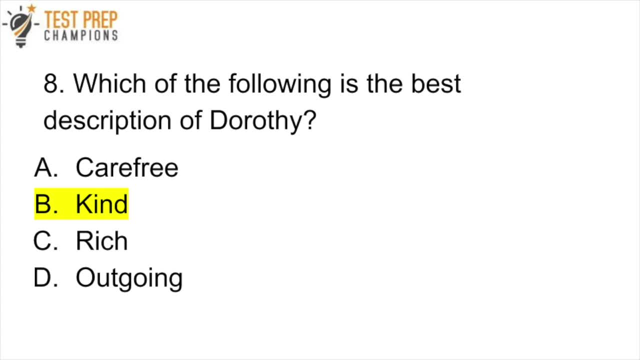 So she does multiple kind acts for the scarecrow. She helps him by, she helps him up and she helps him by offering him food, even though he can't eat it. So since there's multiple acts of kindness by Dorothy, we would conclude that she is kind here. 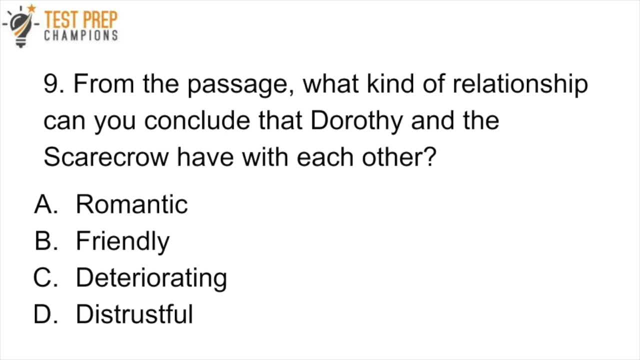 So nine reads from the passage. what kind of relationship can you conclude that Dorothy and the scarecrow have with each other? A romantic, B, friendly, C, deteriorating or D, distrustful? Pause the video and try this out on your own. All right, let's go over this, This type of question. 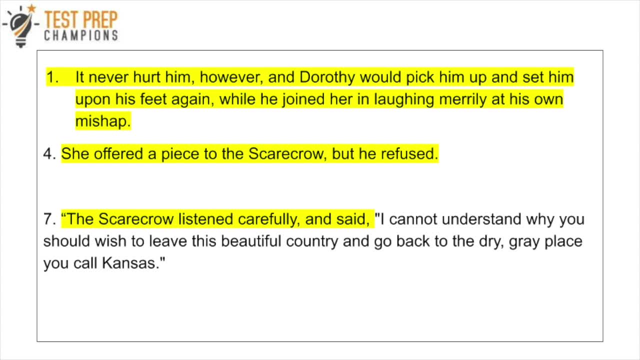 is really important to understand how to do for your test. So, first of all, whenever you're reading a fictional piece on the GED test- fictional is just a word for not real, like basically a story, All right. So when you're reading a fictional piece on your GED test, pay really close attention. 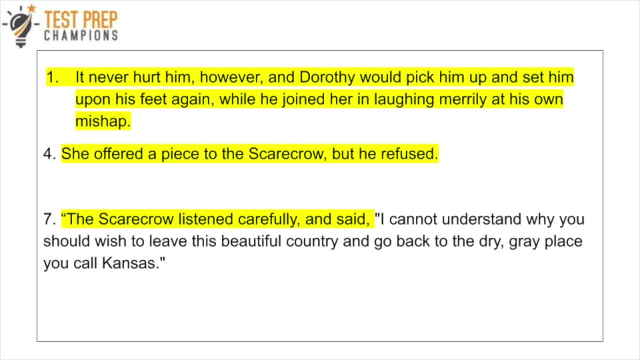 to who the characters are and definitely watch for interactions between the characters So you can always look for the dialogue right. Dialogue is just a fancy word for characters talking in a story, So when you see dialogue in a story, pay close attention to it, because 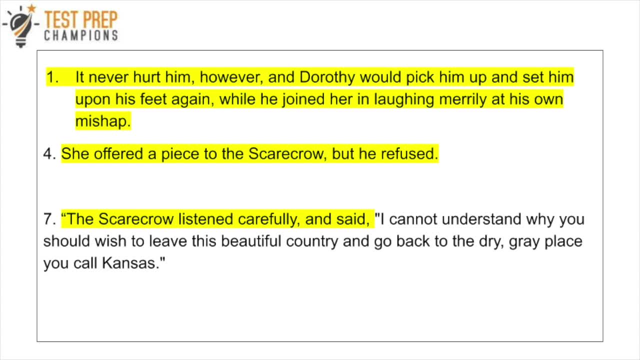 there's a good chance, you might need to use it to answer the questions. So the dialogue is going to help you understand the events and conflicts in the story. Now, when you've got multiple lines of dialogue, note that the start of each paragraph is going to tell you that a different character. 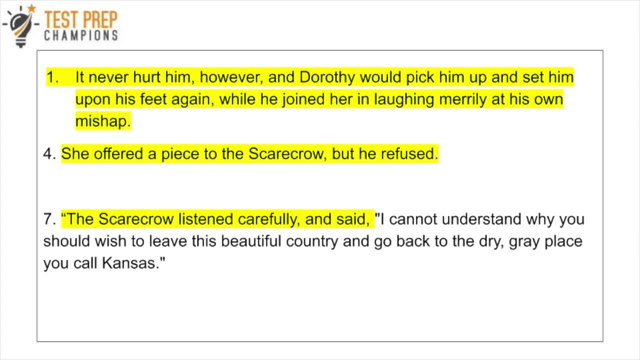 is speaking All right. So to get this question right, we've got to look at the dialogue between Dorothy and the scarecrow. So we're going to look at the dialogue between Dorothy and the scarecrow. We've also got to make some inferences here. So first of all, remember when Dorothy helps up the 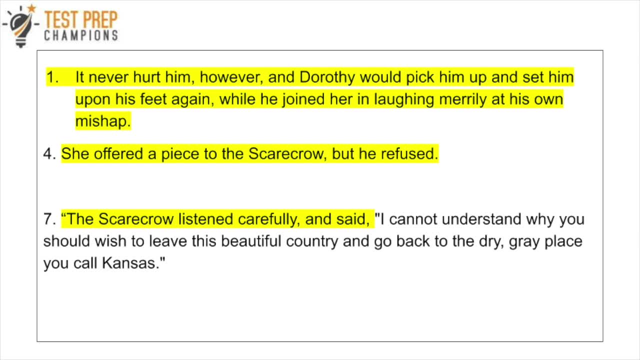 scarecrow, like we just talked about in the last question, and also keep in mind the fact that she's offering him bread. So these are things that a friend would do. So this points to evidence that the relationship is friendly, All right. But more importantly, look at some of their dialogue. So 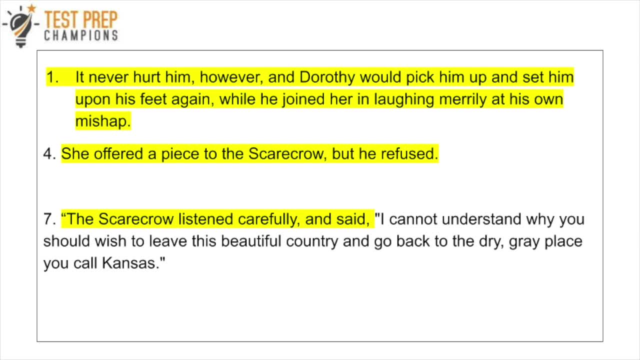 I've just picked out a snippet of it. Look at paragraph seven, where she says: the scarecrow listened carefully. Now, I've highlighted the listen carefully because that's something that a friend would do, right. So we don't see any clues to indicate that they have romantic. 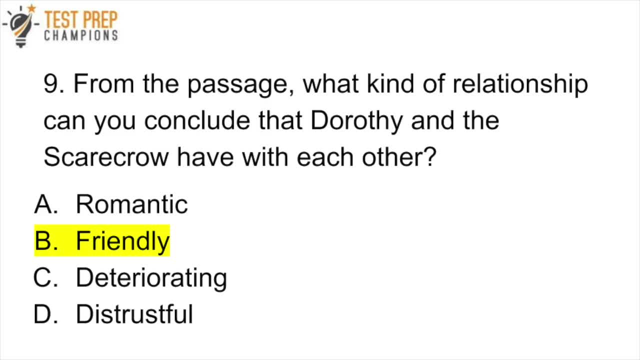 feelings here, right. So there's no handholding, there's no kissing, there's no inferences that we can make. really, that would be logical to say that there's anything romantic going on between them here, So that one is out. So there are also no clues that the relationship is distrustful, All. 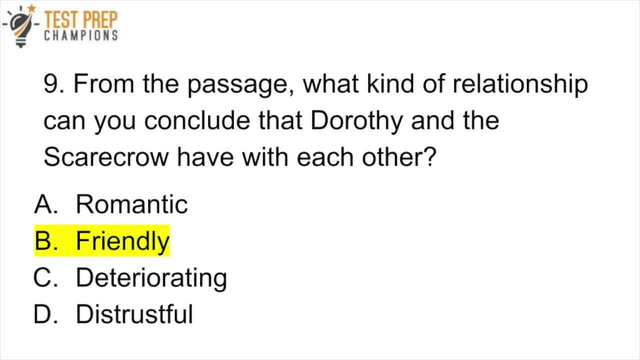 right, Or that the relationship is deteriorating. So deteriorating is a big word, meaning falling apart. So we don't see any indications. In fact, we see things like Dorothy helping the scarecrow, We see the scarecrow listening carefully, a conversation going back and forth between the 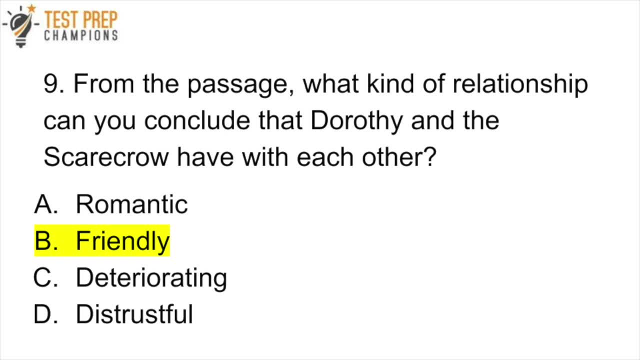 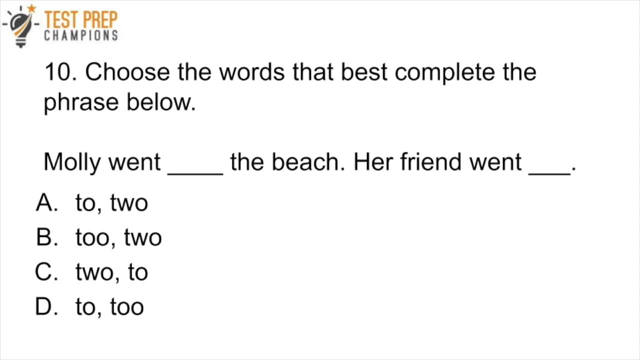 two. So that is something that friends would do here. So by process of elimination we can identify the answer, that the correct answer is going to be friendly. So answer B is right. All right, Moving along to question 10.. Choose the words that best complete the phrase below. 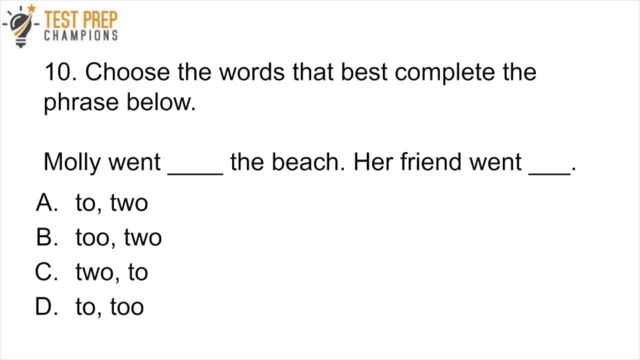 Molly went to the beach Her friend went to. So the challenge here is to pick which forms of the word to do you want to use in each blank. So pause the video and try to figure this out. All right, Let's go over number 10 here. So understanding how to use words that sound the. 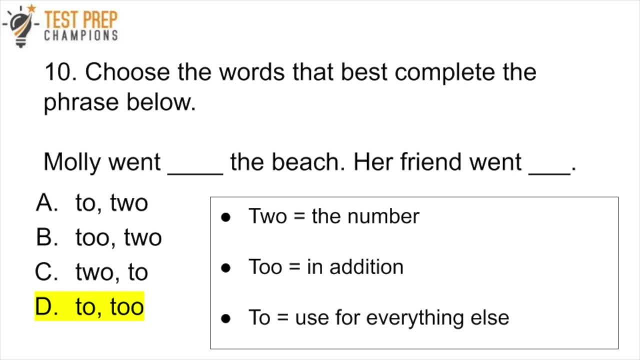 same but are spelled differently correctly is very important for your test And also it's important for the multiple choice questions, but also for your essay, And you can get penalized on your essay if you do this incorrectly here. So the twos are very important to understand. 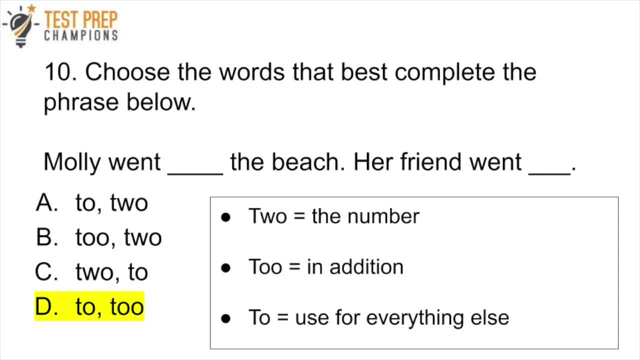 And there's three spellings of two here, So which ones are right? So let's let me break down when to use each spelling of the word to here. So you want to use to spelled TWO when you're talking about number two. Now, to spelled TOO means in addition or also, And to spelled TO is. 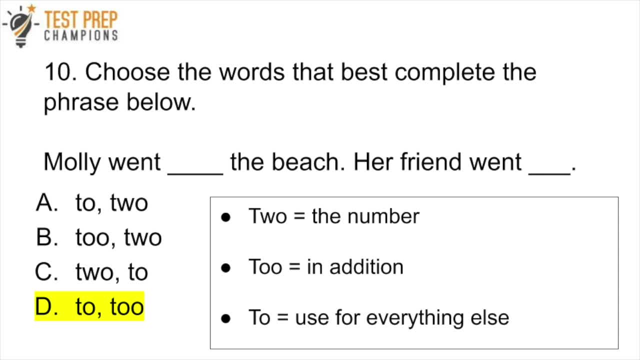 for everything else. So some examples of to spelled TO would be to indicate movement in a direction or a place of arrival. So, for example, she went to the beach. All right, Molly went to the beach. That would be an example of a case when you'd want to use to. 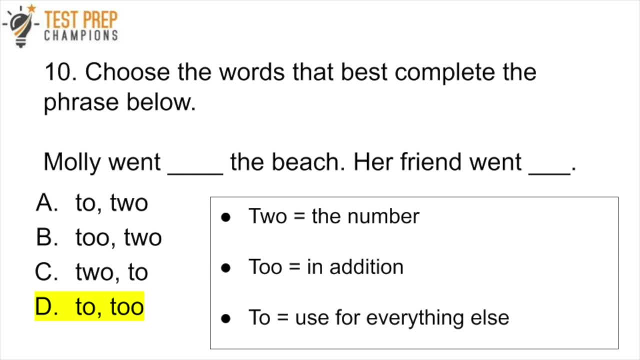 spelled TO. You could also use to spelled TO to indicate a range of time from one o'clock to two o'clock. I'll be doing a live stream. for example, We know that D is the correct answer, So to spelled TO is the first to the second one. 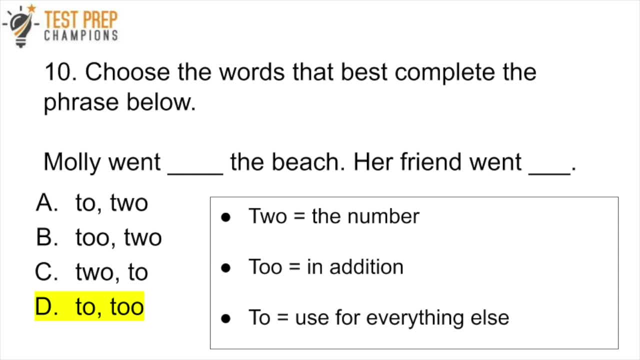 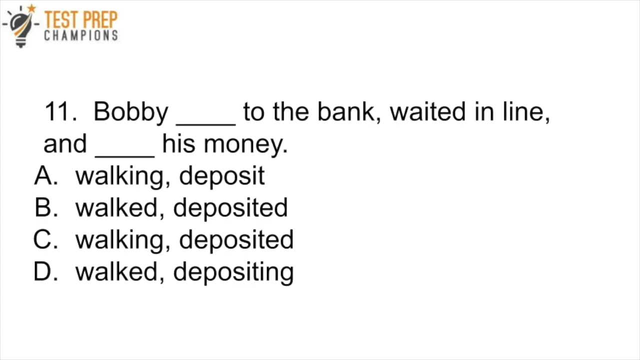 her friend went to. We want to use to, because that means in addition or also. So make sure that you understand how to use these twos correctly, because it is important for your test. So question 11 reads: Bobby blanked the bank, waited in line and blank his money. 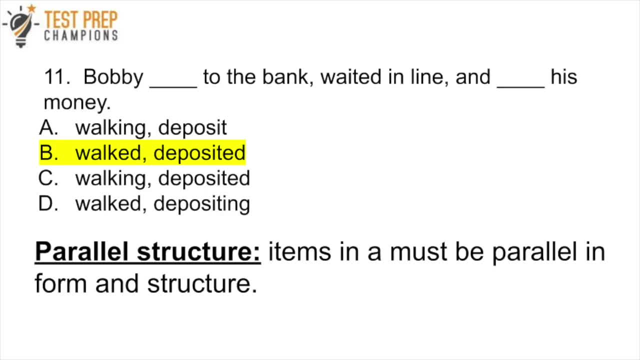 Choose the correct answer- A, B, C or D- and then we'll go over it. So the correct answer here is B. In the sentence you read: Bobby walked to the bank, deposited his money. So a quick trick to answer these kinds of questions is just read them either. 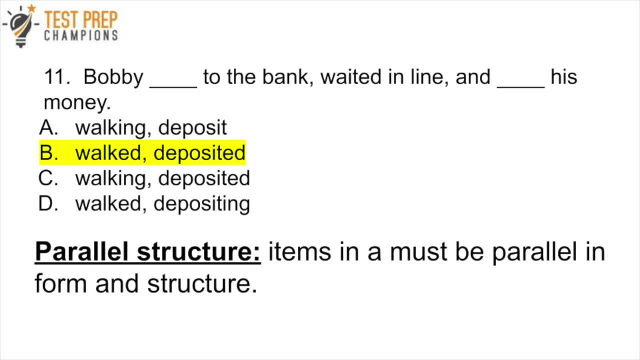 out loud or in your head On your test. preferably do it in your head, obviously, and just see if the sentence sounds right. And the more that you practice reading every day, day by day, you'll get better at just intuitively judging if a sentence is right or not. And you can do this by 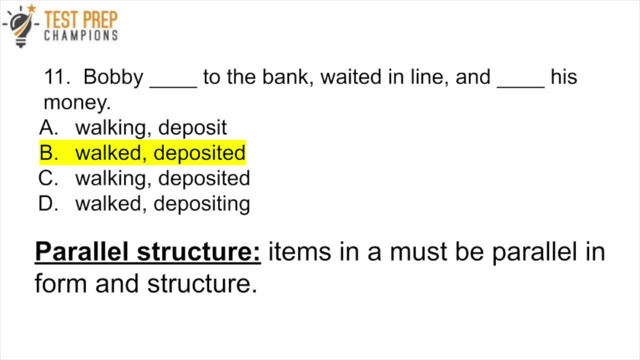 just grabbing an article, reading an article on your phone or the newspaper, or grab some books, whatever it is, Just try to make some time to read. even if it's just 15 minutes here or there, or an hour here or there, It's definitely going to add up and help you get these questions right. 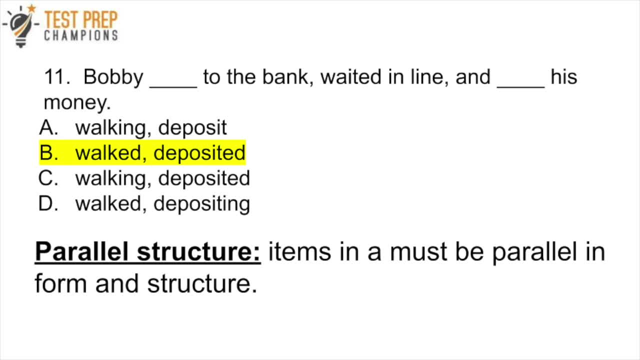 just by using your intuition, But from a language arts perspective, let's dive a little deeper here. So the concept we need to know is parallel structure. So items in a list must be parallel in form and structure. When an author writes a sentence with two or more words or phrases, each word or phrase in the list should be: 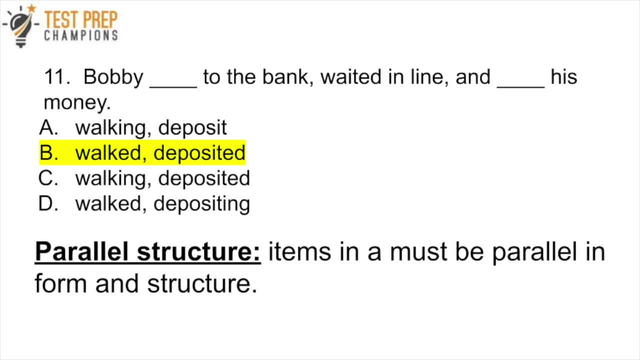 in the same form. So in order to get this right, we want to look at the words like weighted here. The word weighted is a clue here, And if you want to learn more about verb forms and verb tenses, you'll want to watch my video on GD grammar lessons. I'll put a link to that down below. 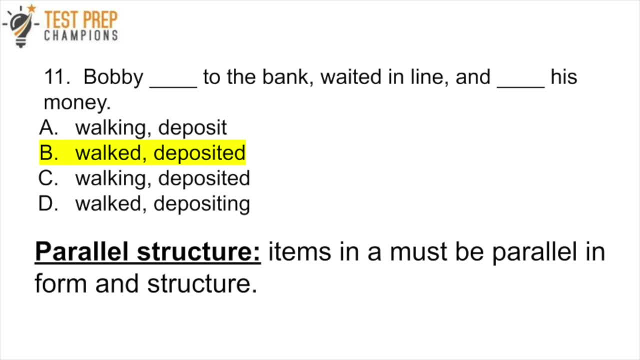 I explore that concept in depth. But basically we just want to understand that walked and deposited are going to be correct And we see that walk in deposit right. if we add ED to both of these, we're going to have the same. 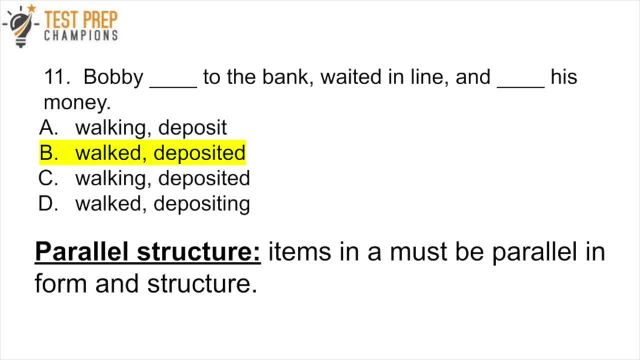 form as: weighted right. Weighted the word weight, they put an ED on it for the sentence. So that's kind of your clue to get this right. And also note that in a list like this the commas should separate the words or phrases. So Bobby walked to the bank. comma: weighted in line comma. 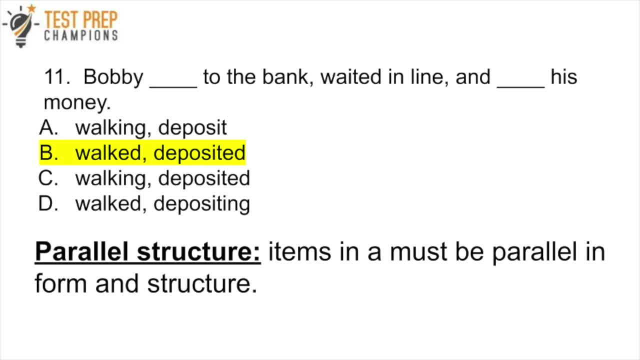 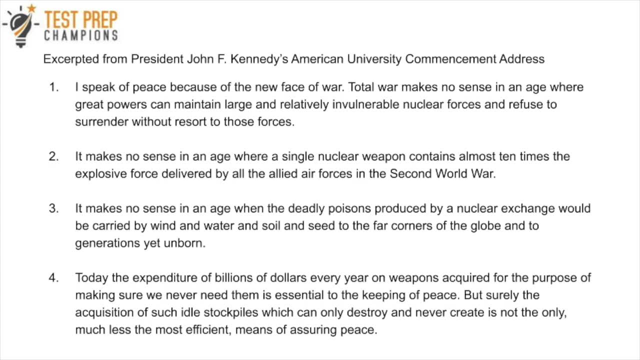 and deposited his money, All right. And so again, it's that ED at the end of weight, It's the ED at the end of walk, the ed at the end of deposit, right, That's the key to getting this question right is seeing that. Okay, here's another example of a passage. So we're going to test. 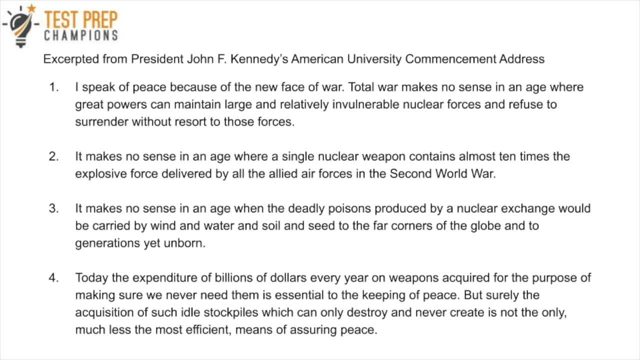 your reading comprehension skills now. So this is excerpted from President JFK's American University commencement address, And let me just get right into the excerpt here. So he says: I speak of peace because of the new phase of war. Total war makes no sense in an age where 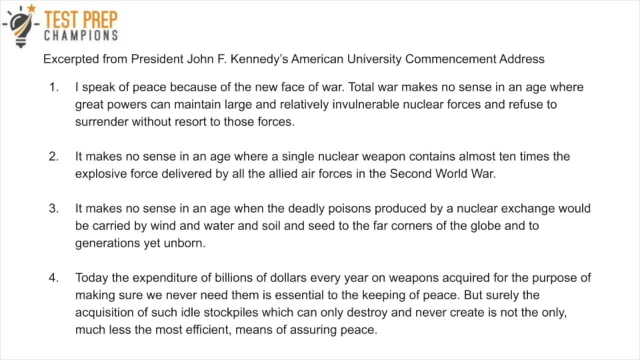 great powers can maintain large and relatively invulnerable nuclear forces and refuse to surrender without resort to these forces. It makes no sense that, an age where a single nuclear weapon contains almost 10 times the explosive force delivered by all the allied air forces in the Second World War. It makes no sense that an age when the deadly poisons 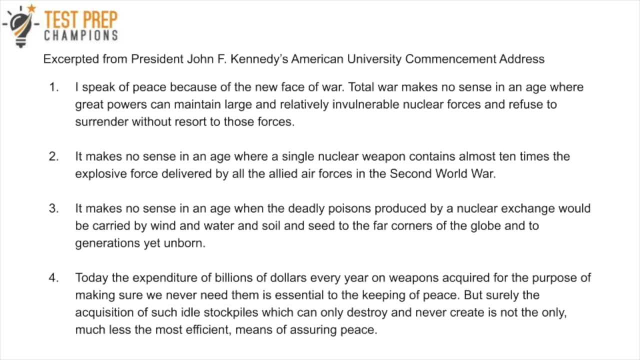 produced by nuclear exchange would be carried by wind and water and soil and seed to the far corners of the globe, to generations yet unborn Today. the expenditure of billions of dollars every year on weapons acquired for the purpose of making sure we need- we never need them is. 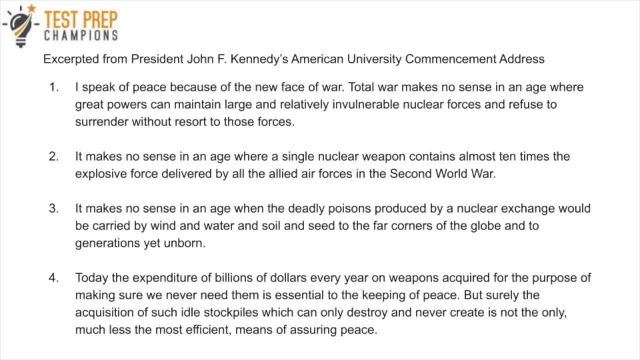 essential to keeping the peace. But surely the acquisition of such idle stockpiles, which can only be achieved by the use of weapons, is essential to keeping the peace? Only destroy and never create is not the only, much less the most efficient means of assuring. 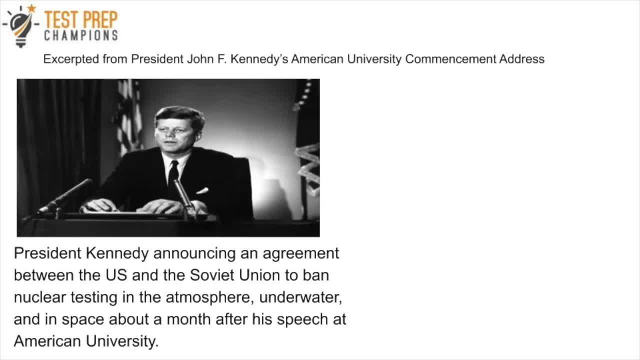 peace. Okay, so that's the excerpt. And along with this excerpt we see there's also a picture and there's a caption below the picture which gives us some extra information. So the caption reads: President Kennedy announcing an agreement between the US and the Soviet Union to ban. 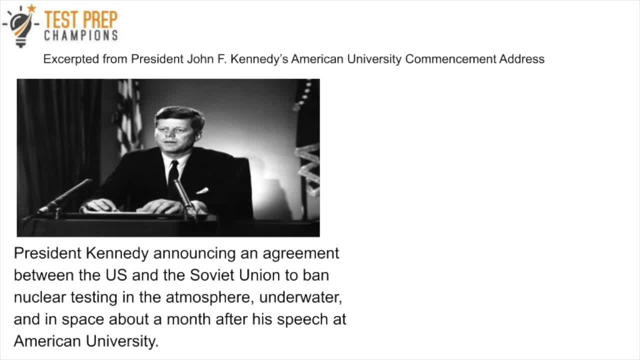 nuclear testing in the atmosphere, underwater and in space about a month after his speech at American University. So, as always, you can pause the video, rewind, whatever you need to do to read that passage in full. And now we're going to move on to the questions. 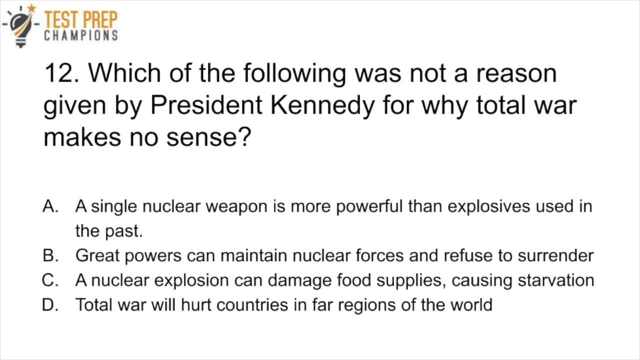 So question 12 reads what's the following: what's not a reason given by President Kennedy for why total war makes no sense? A- a single nuclear weapon is more powerful than explosives used in the past. B- great powers can maintain nuclear forces and refuse to surrender. C- 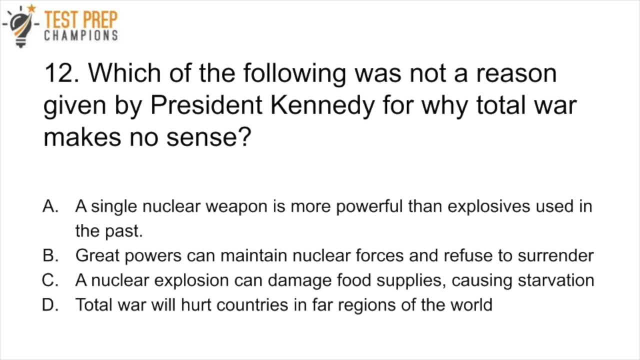 a nuclear explosion can damage food supplies, causing starvation. Or D- total war will hurt countries in far regions of the world. Go ahead, pause the video. you know the drill. So the correct answer to number 12 is C- a nuclear explosion can damage food. 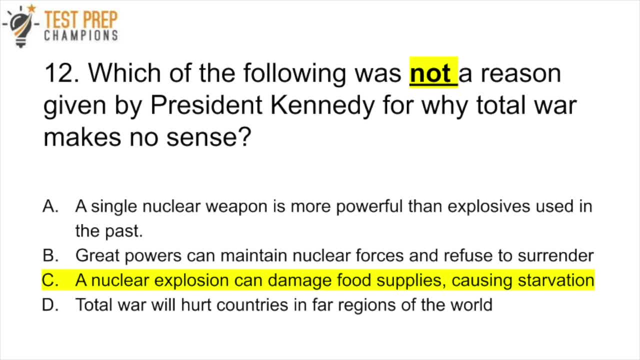 supplies, causing starvation. So this may or may not be a result of nuclear war or total war, but we don't see any evidence for this in the passage right. So in the excerpt that we read, President Kennedy did not cite this as a reason. All of the others- A, B and D- were reasons given. 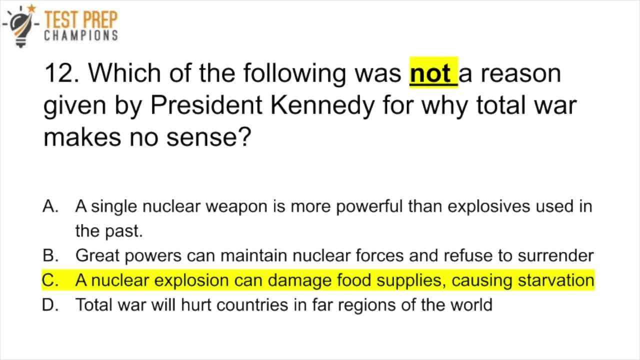 by President Kennedy for why total war makes no sense, And so I've highlighted and underlined and bolded the word not here, because whenever you see the word not, you always want to pay close attention and make sure that you are answering the question. which of the following was not a reason? 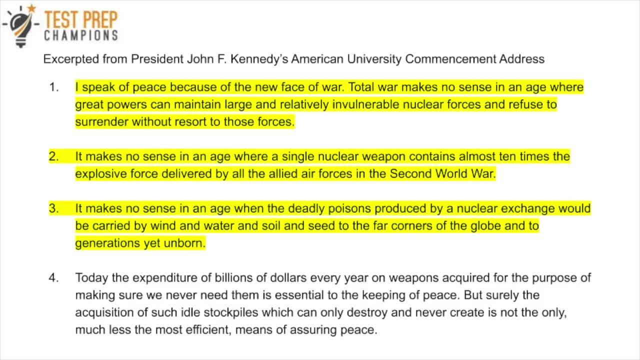 not. which of the following is a reason. So if you have trouble with this question, let's look at the passage again quickly here. So we see that answer choice C was not included here in the passage by President Kennedy and we can find A, B and D in the highlighted portions here at the passage. So it's really. 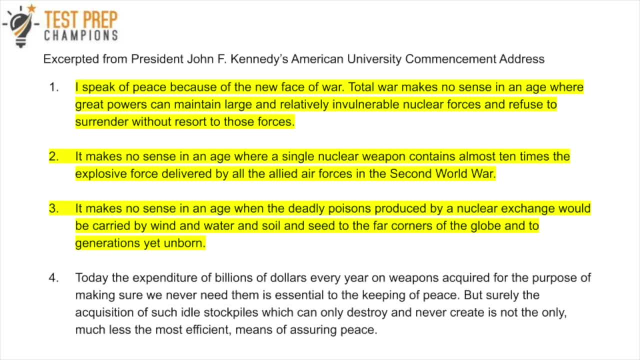 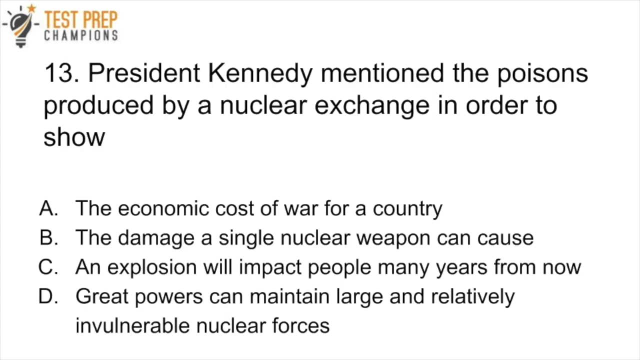 important to just get in the habit of reading these passages and then going back to the passages as needed. Or you can rely on your memory too, but it's always good to just double check the passage and confirm Question 13,. President Kennedy mentioned the poisons produced by nuclear exchange. 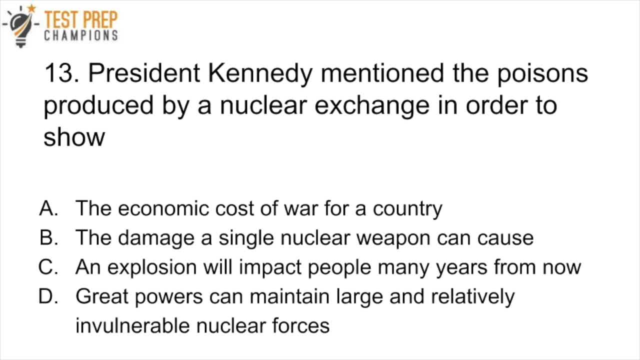 in order to show: A- the economic and economic benefits of nuclear weapons, B- the economic and economic cost of war for a country, B- the damage a single nuclear weapon can cause. C- an explosion will impact people for many years from now, Or. D. great powers can maintain large and relatively. 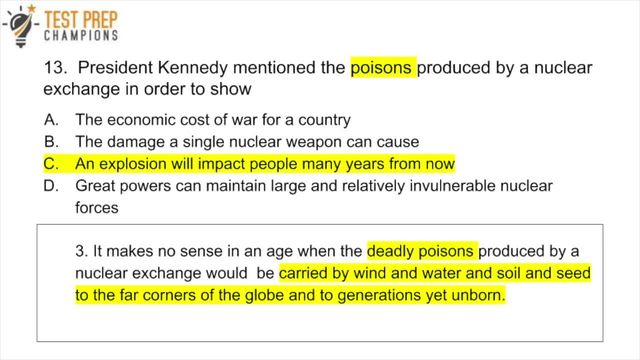 invulnerable nuclear forces. Pause the video and give this one a shot. So the correct answer is C and this comes right out of the passage from paragraph number three. So in the question I've highlighted the word poisons, because that's really your key word here. So we want to look at. 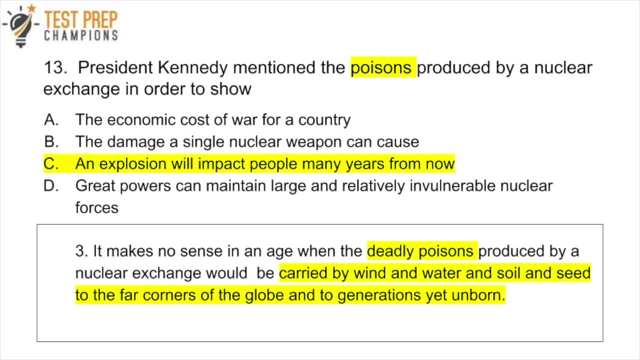 the passage in paragraph number three. It makes no sense in an age when the deadly poisons produced by nuclear exchange would be carried away. So we want to look at the passage in paragraph number three. So answer C: an explosion will impact people many years from now. When it says in the: 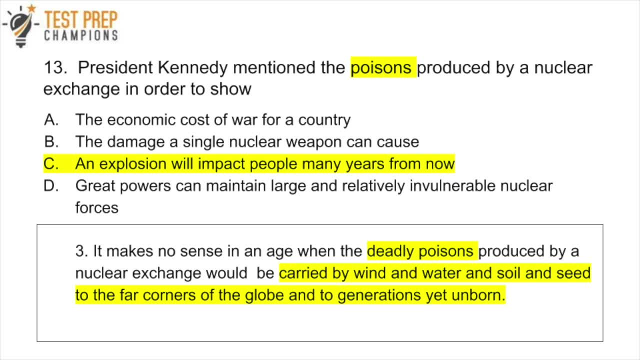 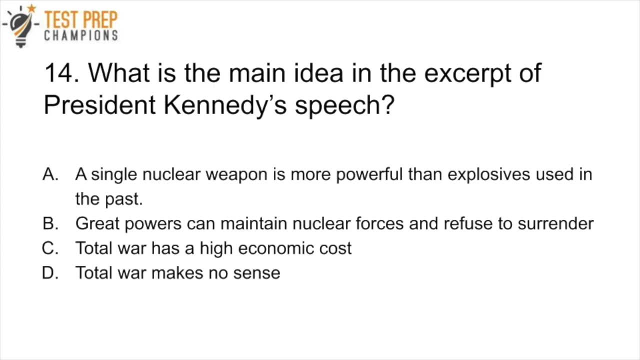 passage generations yet unborn. that's talking about people that are going to be born many years from now. So that's why answer C is correct. Number 14,: what is the main idea in the excerpt of President Kennedy's speech? A: a single weapon is more powerful than explosives used in the past. 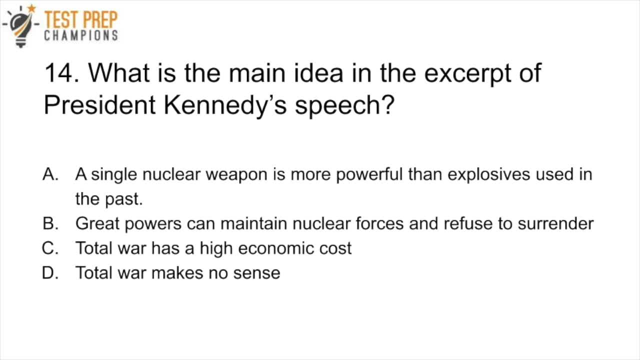 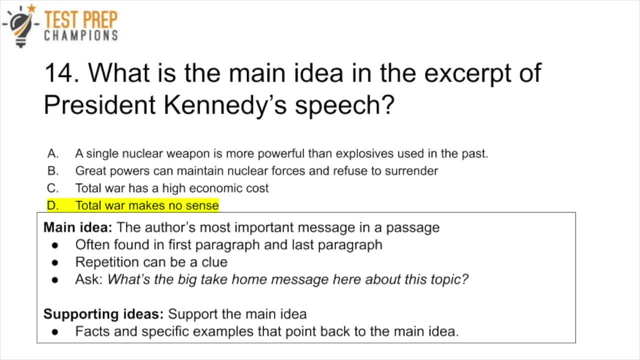 B- great powers can maintain nuclear forces and refuse to surrender. C- economic cost Or D- total war. makes no sense. Pause the video and give this one a try. So D is the main idea. A, B and C are specific examples given to support the main idea. So A. 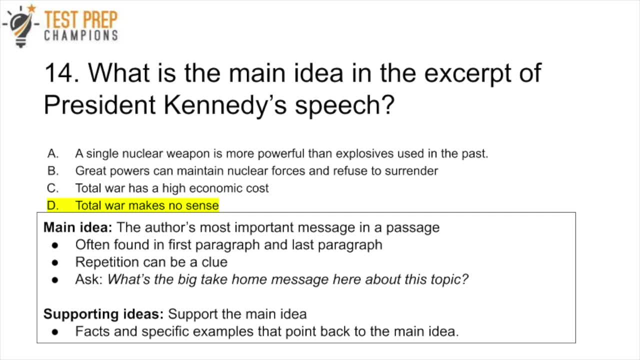 B and C are supporting details, And what we have to understand here is the difference between main ideas and supporting ideas. okay, So really the main idea here is the author's most important message in the passage, And this is often found in the first paragraph or in the last paragraph. 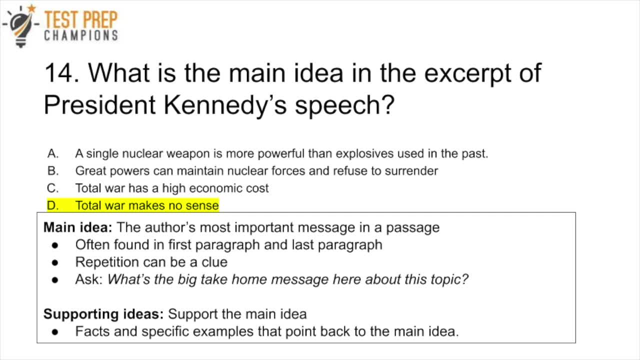 although in this example that's not the case- And another way to find the main idea is to look for repetition. So sometimes the author is going to directly state the main idea several times, or they might imply it several times, sometimes in multiple different ways. 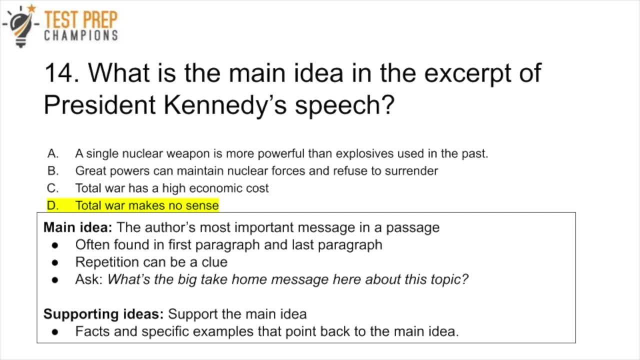 okay, And another great way to do it is to just ask, as you're reading, what's the big take-home message here about this topic, Or what's the author's point here, And so kind of a secret trick for really quickly identifying the main idea is to just imagine that you're the writer. 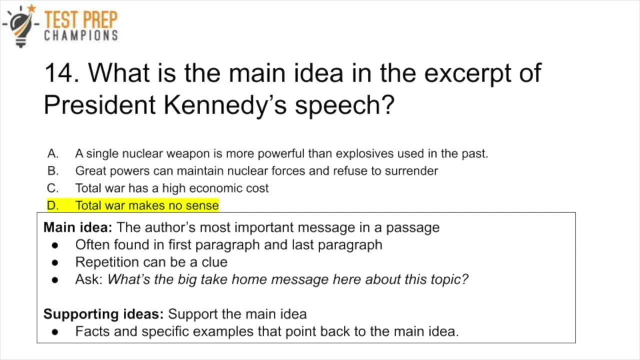 and you have to write a headline or your own title for the speech. What would you call it? All right, And so often that question can kind of clue you into what the main idea is, because you're condensing, you're taking the whole passage and you have to think. 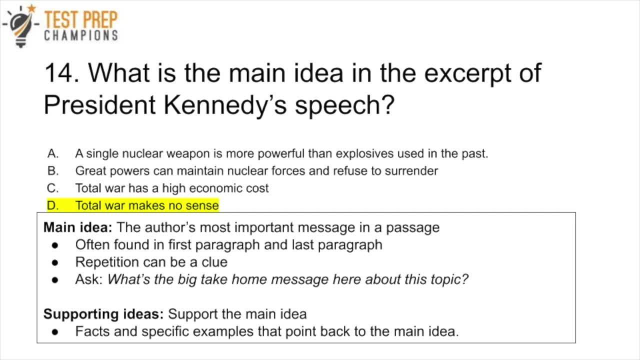 hey, in just a few words, what would I title this? okay, And by doing that, that's often going to cause you to focus in on what the main idea is. So, also, you want to be aware of supporting ideas, and supporting ideas support the main idea. So these can be things like facts, specific. 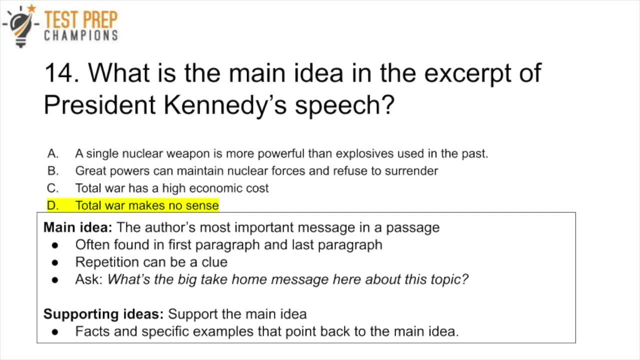 examples, details, other arguments that are being used by the writer, that all point back to the main idea. So the difference here is main idea versus supporting idea, and D is the main idea here And the main idea will be a more general statement, whereas the supporting ideas are going to be more. 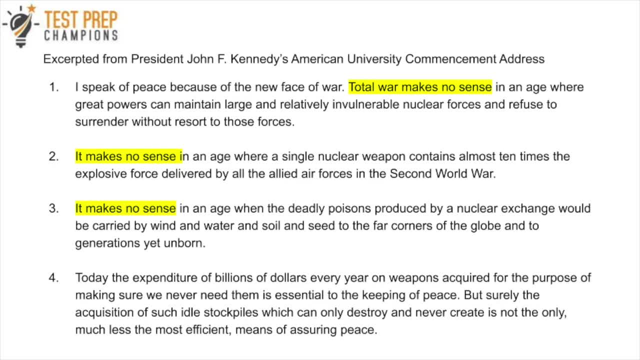 detailed and will be more specific examples. So just to help you understand what I mean by repetition, I've highlighted a couple times where President Kennedy used repetition here, followed by examples. So he says total war makes no sense in an age where great powers 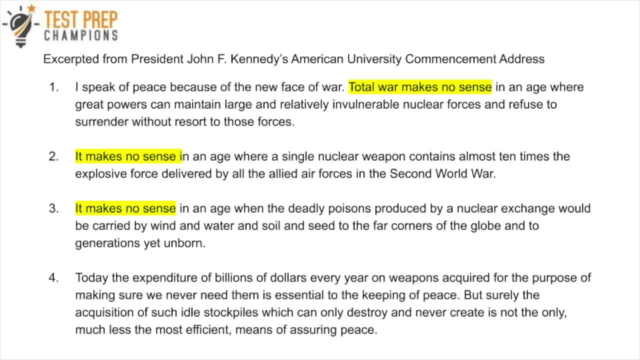 blah, blah, blah, blah, blah. In number two: it makes no sense. blah, blah, blah, blah, blah. In number three: it makes no sense. blah, blah, blah, blah blah. So we see that repetition here. 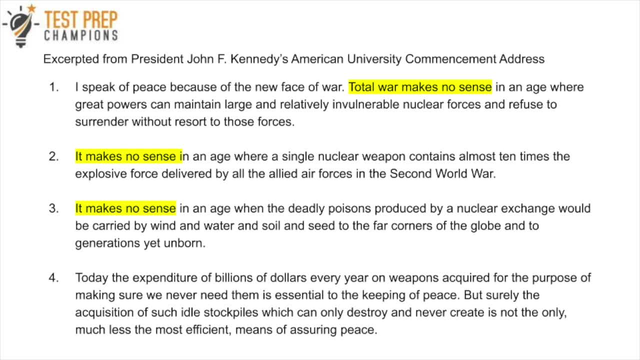 and that helps us understand that the fact that total war makes no sense is the main idea. And then, following the main idea, he gives supporting examples that show that there's a lot of damage here, right? So, following the portions that I've highlighted are: 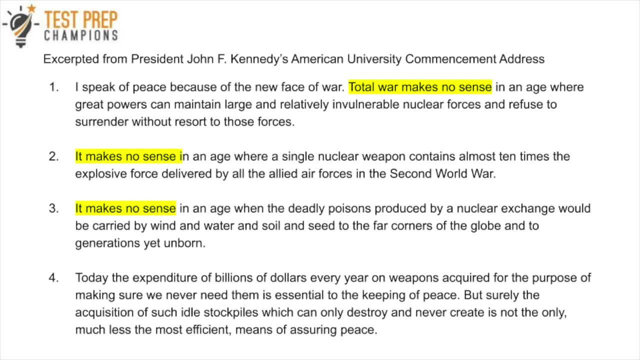 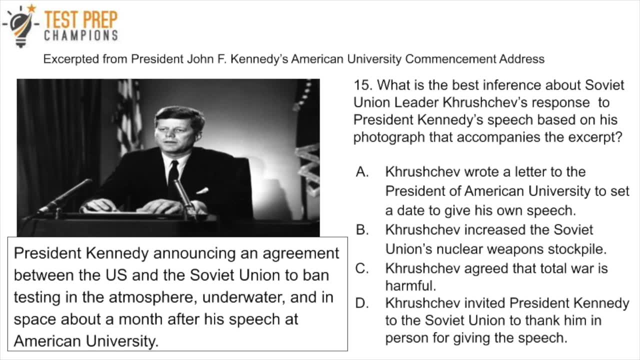 detailed examples that show why there's damage and support, why total war makes no sense. So in question 15, we see that we have another question, that, and this time we have a question about that photo. So 15 reads: what is the best inference about Soviet Union leader Khrushchev's? 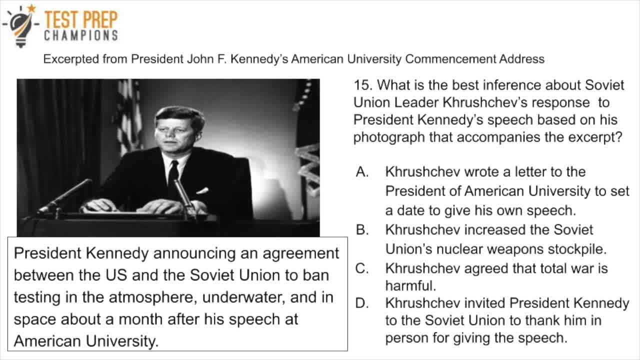 response to President Kennedy's speech based on the photograph that accompanies the excerpt. You can see the excerpt. we read it earlier. pause the video and try to solve this question here, But just know that this is fair game. you may get questions on your test that give you photographs with with a caption below. 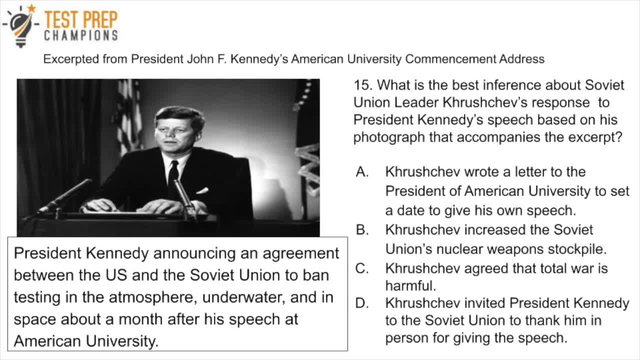 and a caption may mention something or hint to something that was not explicitly stated in your passage, but it's going to extend the information in the passage, So pause the video and try to answer this. The correct answer here is C, And so this is another one. 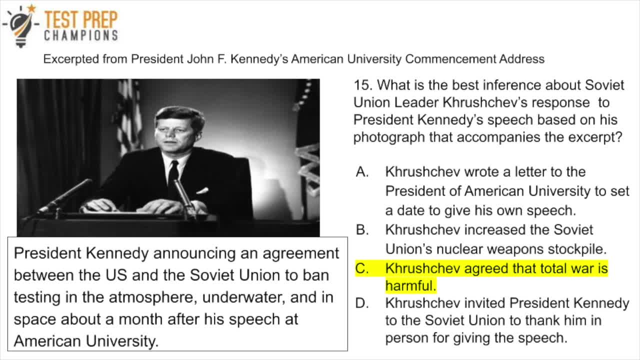 of those inference questions And it's really just a common sense, logical question, right? So remember, an inference is just an educated guess that you make based on the information that you're given. So that's the first thing that you want to do is look at that information. 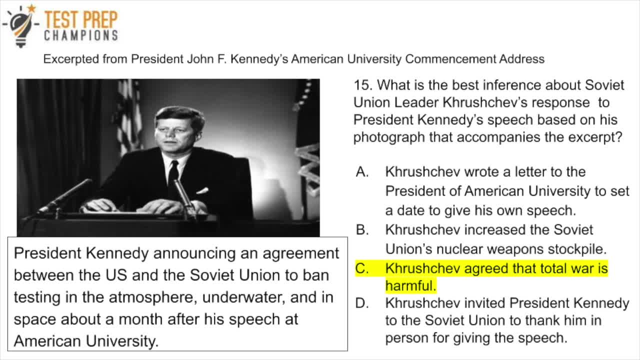 that you're given here And then you just have to use some logic and you have to use some common sense here and don't overthink these questions, right? So we have to consider the main idea in that speech And we have to think about the text, right? Think about. 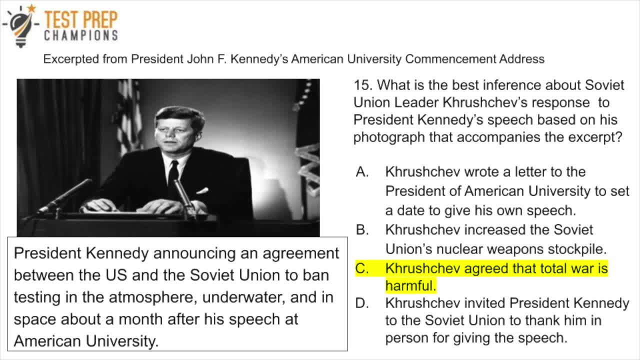 that excerpt. we might need to revisit that excerpt And also we want to look at the photograph and look at the caption and think about the information that we're told here. Okay, so the so remember, the theme of that speech, or the main idea of Kennedy's speech, is that 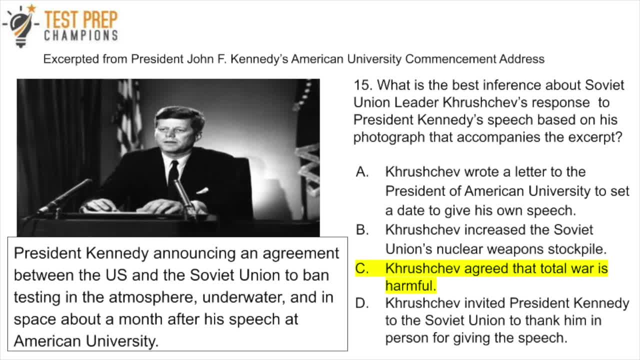 total war is bad and peace is good, basically right. And so this caption here underneath is telling us that there was an agreement reached by the US and the Soviet Union to reduce certain types of weapons testing. Okay, and we're also told, which is really the key- 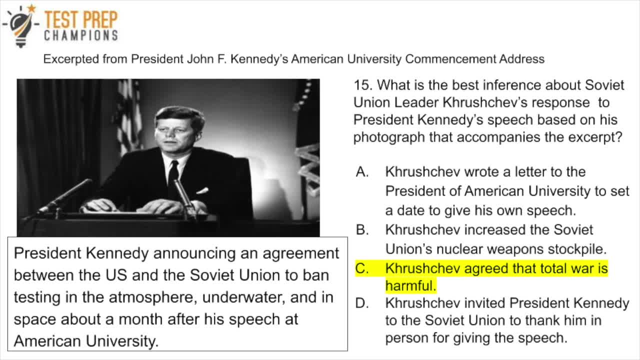 piece of information here that this was about a month after his speech at American University. Alright, so we can kind of make a, an educated guess about a cause and effect relationship here, right, And so if we really think about this effect here, so what is the effect here? 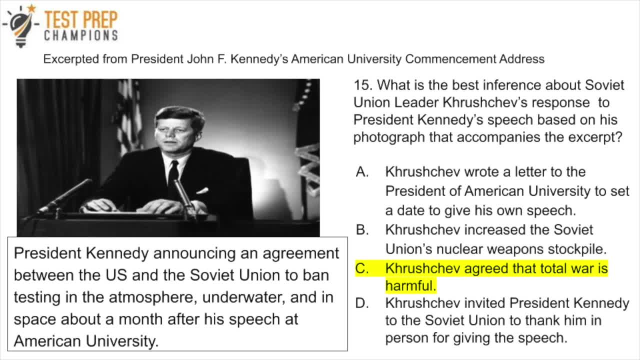 the effect is that there was an agreement reached, okay, between the US and the Soviet Union that would reduce certain types of weapons testing. Alright, so now let's think back to that And think: well, if that was the effect, what was the cause? Well, since we're told that, 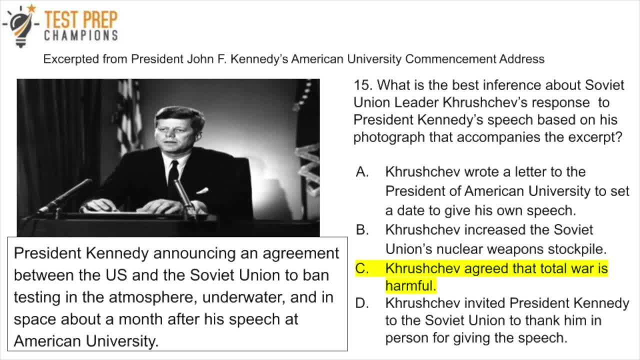 Kennedy gave a speech a month before this agreement was reached, then we can kind of infer here that, hey, that was a cause, or at least one of the causes, right, So there may have been multiple causes here. there may there probably was multiple contributing. 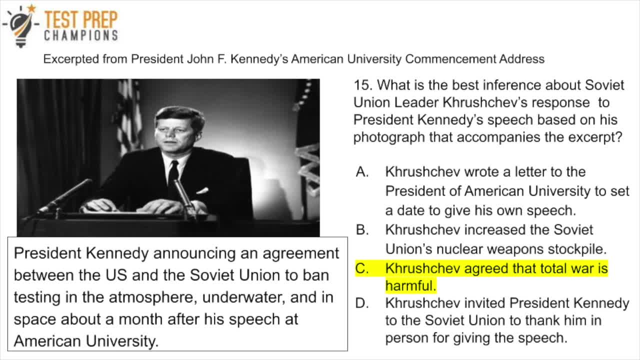 factors that led to this agreement being reached, but one of them would have been the speech, And that's kind of what we want to think logically here. we want to put two and two together between the fact that this speech was given- we know that the main idea was was peace- and 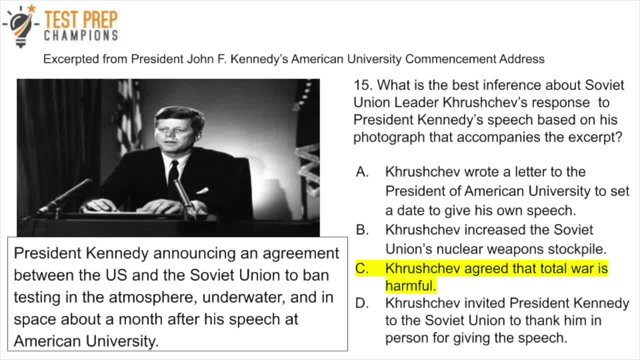 why total war is bad. And then we see that about a month after the agreement was reached and then we see that about a month later there was a peace agreement reached between two countries. So we've got to first make that connection here And we've just got to use logic in the process of elimination. 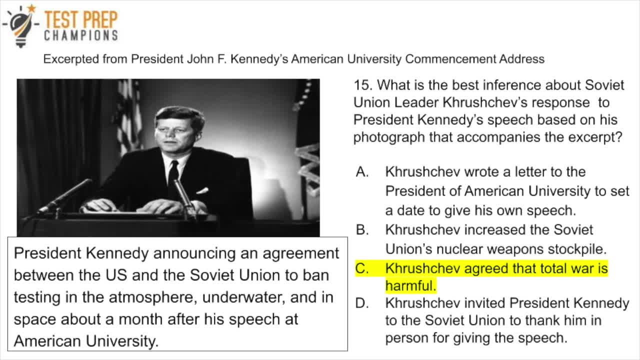 So a Khrushchev wrote a letter to the President of American University. he said a date to give his own speech. Now, this may or may not have happened. Okay, now, historically we know that this never happened because Khrushchev never spoke at American University. 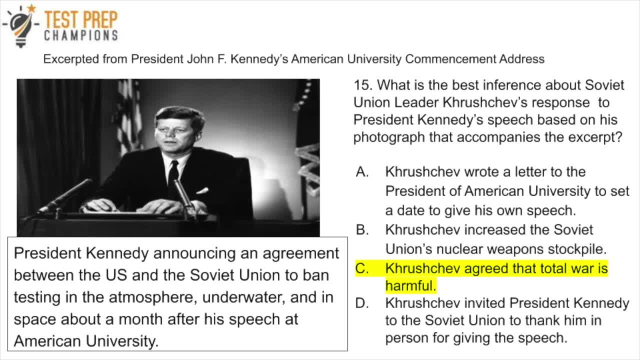 But you don't have to know any historical facts here, right? This is language arts, this is reading comprehension. So just from common sense perspective here, is there anything in the passage that would hint that a would be correct? No, I don't think so. Same with: 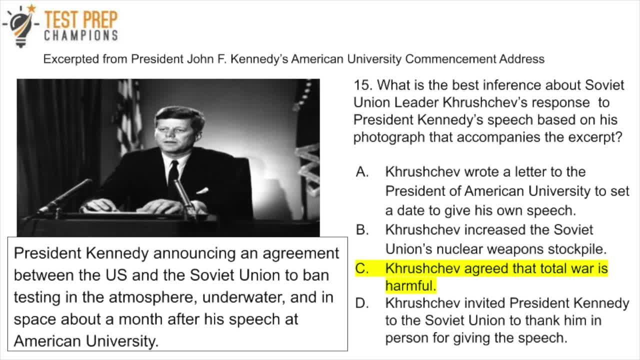 B Khrushchev increased the Soviet Union's nuclear weapons stockpile. So we just have to use logic here, right? So if we look at what the caption tells us, the caption is telling us that the Soviet Union essentially decided to stop testing certain types of weapons. 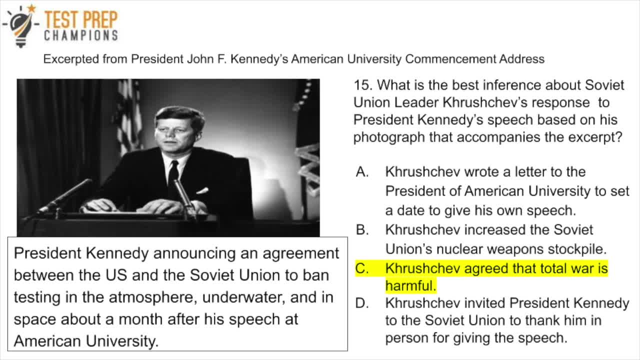 All right, And so if they're banning certain testing, certain types of weapons, chances are they're not also increasing the nuclear weapons stockpile. Now they may or may not have decided to ban testing in the atmosphere, underwater and in space. they might have done. 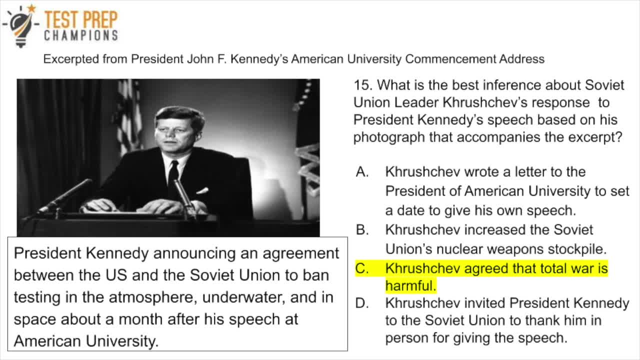 that and then also increase their weapons on land. But we don't know that here, right, That wouldn't be a logical guess based off of the caption and the information in the passage here. And so D Khrushchev invited President Kennedy. 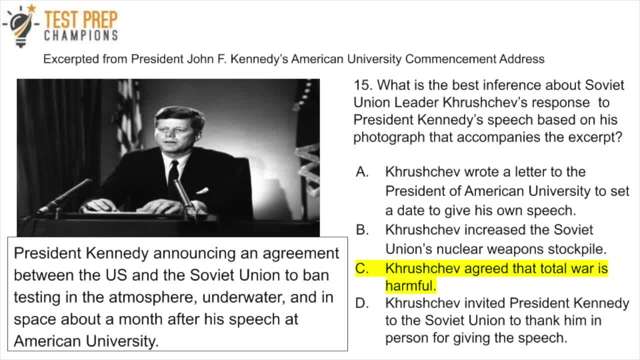 of the Soviet Union to thank him in person for giving the speech. Now, this may or may not have happened, And but just use common sense here. Does that sound like something that would happen? Probably not really, But also, you can use common sense and also look. 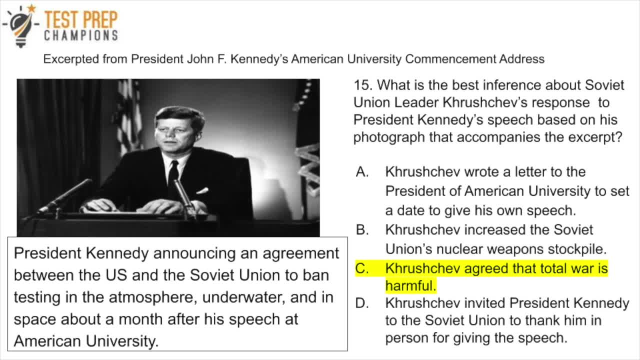 at the details in the passage. Is there anything in the passage or in this caption that would hint that the Soviet Union leader thanked President Kennedy and wanted him to come, come to the Soviet Union in person to give him a big thanks? Well, I don't think that's really. 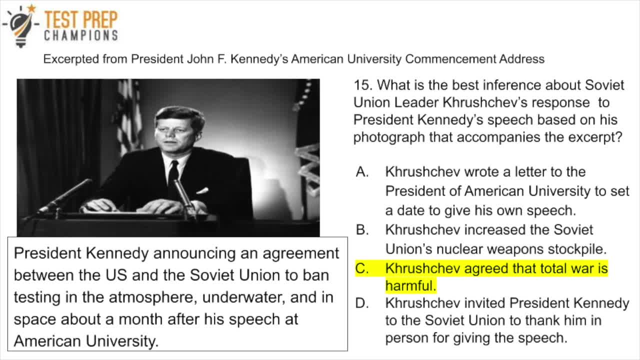 a logical connection, right? So C is the most logical here- that Khrushchev agreed that total war is harmful. And again, we can see this just from the fact that President Kennedy gives this big speech on why total war is bad and why peace is good. Then, about a month, 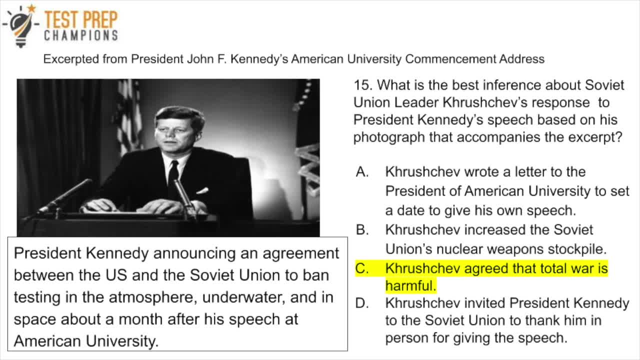 later there's this, essentially a peace agreement reached between the US and the Soviet Union to ban testing of certain types of weapons, And so we conclude that he must have agreed that total war is harmful, because he brought his country to the negotiating table, and this 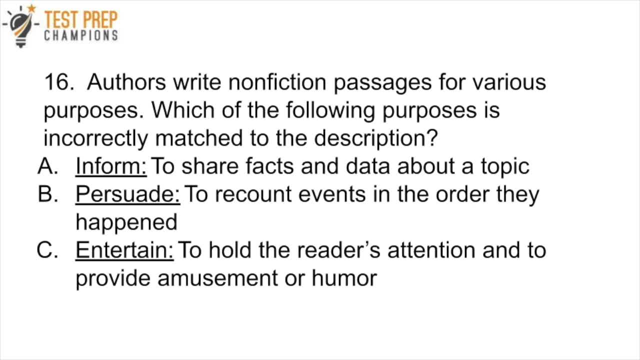 peace agreement was reached. So question 16 reads: authors of the Soviet Union and the US have agreed to ban testing of the Soviet Union. Okay, so the answer is B. So these are some. so first of all, here's just a general tip. 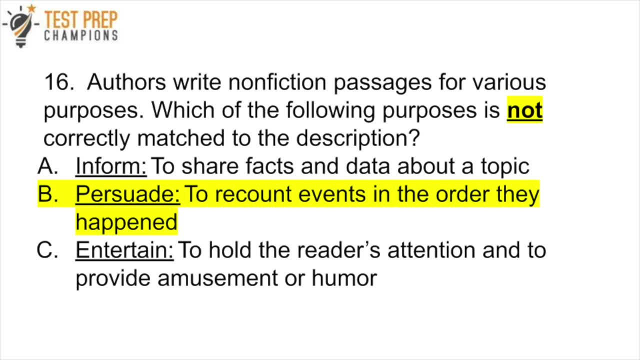 that I want to give here. You want to pay attention to the word not always, and this has been a reoccurring theme throughout the practice test here, but i've highlighted this and emphasized it in order to point out that the word not is so important to spot, because it says which of the following purposes is not correctly: 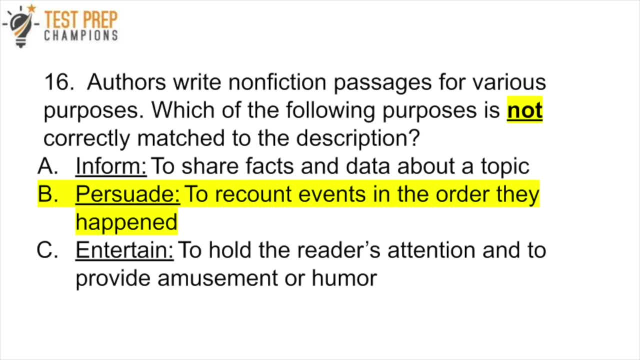 matched to the description. so a trap would be to say which of the following purposes is correctly matched to the description. read a and say, oh hey, a is correctly matched. so therefore, a is the correct answer here, because sometimes, when, especially in the, during a testing condition, when it gets, 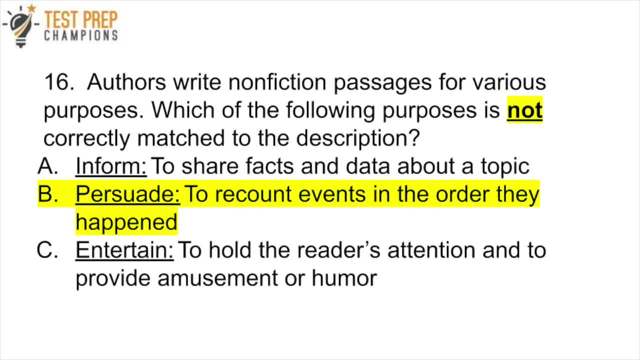 stressful for us or we see that timer ticking down and we start to panic a little bit, we- our brain- will just skip the word not for some reason, when we read. so make sure that you slow down and always read questions and pay attention to the word nots. okay, sometimes it helps to read questions. 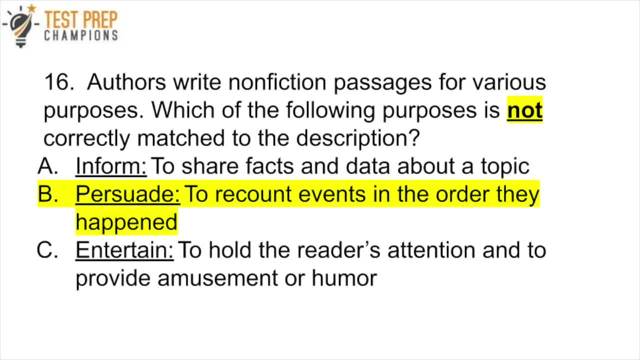 twice. but anyway, an author might write a piece for one or more of these purposes, and it's important to know at least four of them: to narrate, to inform, to persuade or to entertain. so to inform would be to share facts and data about a topic, and this could be like a news article or a science article. 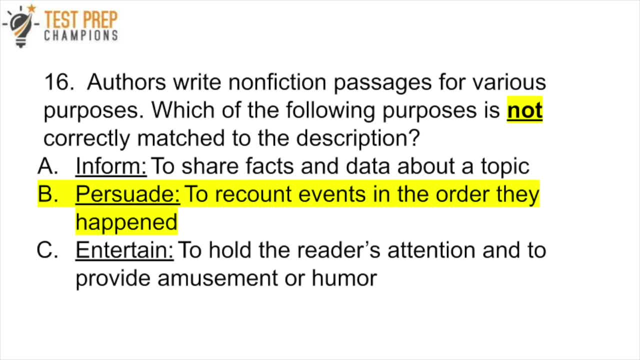 for example, a narrative passage is just like a non-fiction story. it recounts events in a series. so b actually fits the description of a narrative. so to narrate? so if the purpose was to narrate, it would be to recount events in the order that they happened. so that's. 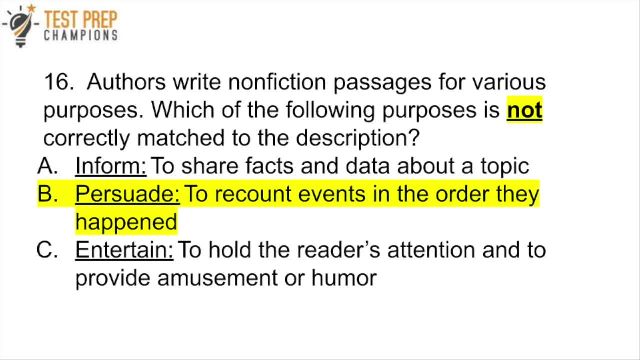 why b is wrong. a persuasive passages is actually when the author wishes to persuade you that their position is correct. so this could be like an opinion piece about, say, politics, or about some kind of social justice issue or about, like an environmental issue. that would be a persuasive. 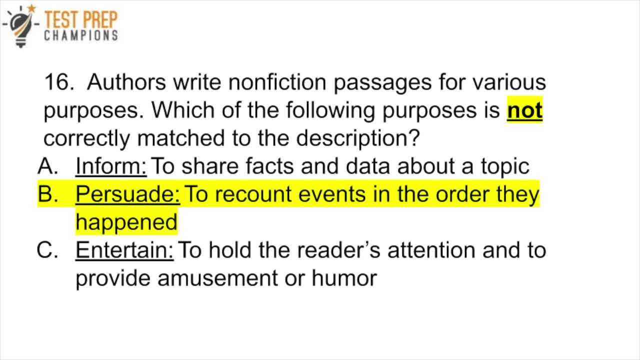 piece when the author wants to change your mind. now, entertainment is something like a comic like- think of like a little comic strip in the newspaper. or it could be like a humorous article or something like that, something that's just there to entertain you and provide amusement or humor. 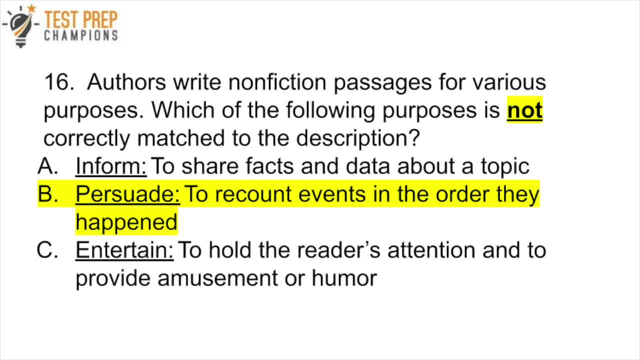 okay, so let's move on here to number 17. so it says experts have mixed opinions on what the best method for working out is. although running and yoga are both beneficial, running burns more calories. however, yoga packs on more lean muscle. so question 17 says: what is the writer comparing and contrasting? 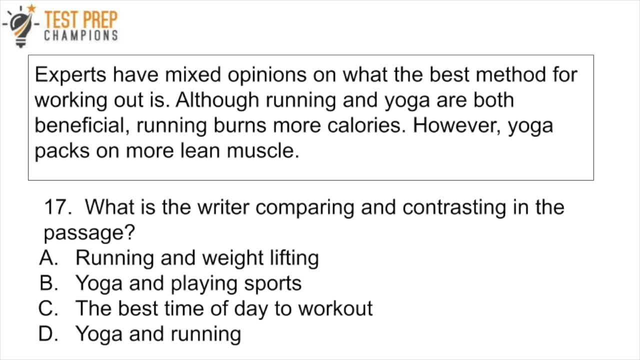 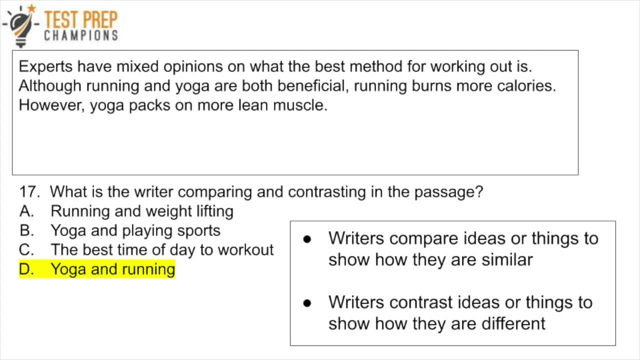 in this passage. so pause the video, read answers a through d and pick whichever one you think is the best and, of course, as always, we're going to go over it all. right now it's time to go over it. so the answer is d: yoga and running here. so you always want to watch out for passages in which ideas or things are compared and 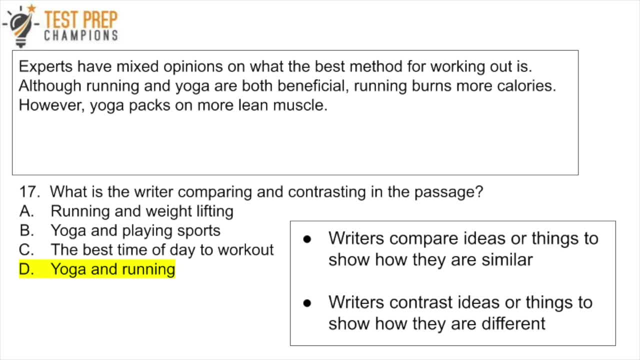 contrasted, so you might get a passage in which things or ideas are compared and contrasted in the same paragraph, as we see here, or you might also see this done over the course of multiple paragraphs and the author could go back and forth between talking about running in one paragraph and 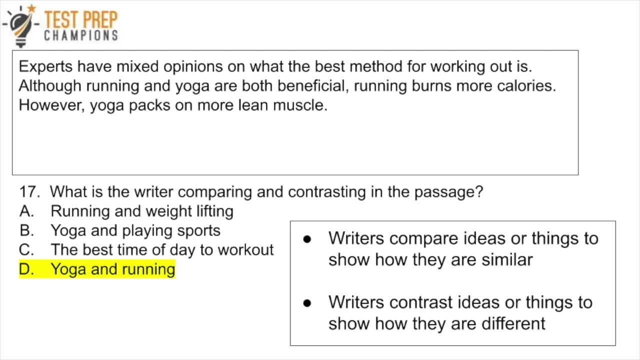 then yoga in the next, then running in, so on and so forth. so you just want to watch for this. okay, writers, compare and contrast and then you might get a passage in which things are compared and contrasted. so again, the correct answer is d: yoga and running are being compared and contrasted in. 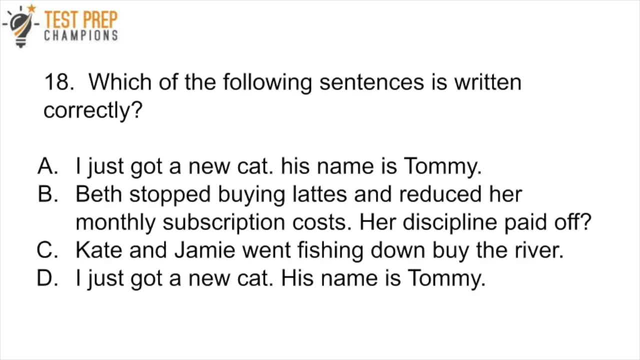 this small little passage here, so let's keep rolling here. let's go on to 18, so which of the following sentences is written correctly? and i'll let you read the answer choices for yourself. so pause the video and let's try to do that now. okay, so let's go over this. the correct answer is d, but 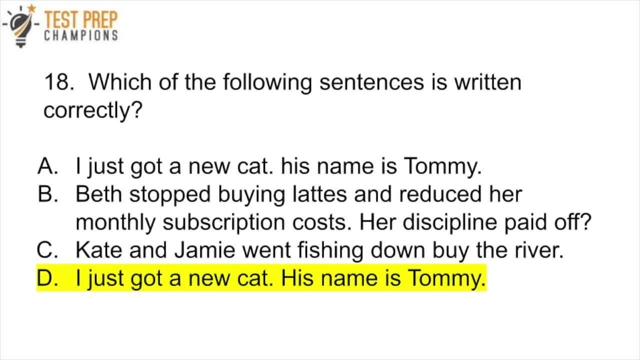 it's really crucial that we break down why each answer choice is wrong. so if you haven't done so already, um, make sure you pause the video again and try to do that again. so let's go over this and try to actually stop and think. why are a, b and c wrong? because a big part of the exercise here. 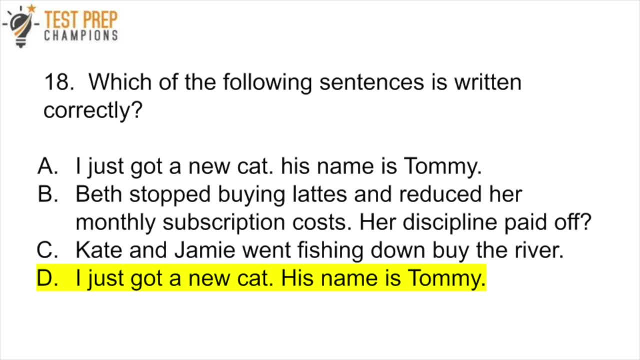 and the learning is not going to take place just from finding the right answer, but as well as identifying why each choice is wrong. all right, so let's go. let's break this down, and there's many, many important lessons here that are really going to help you on the gd, so this is kind of like a 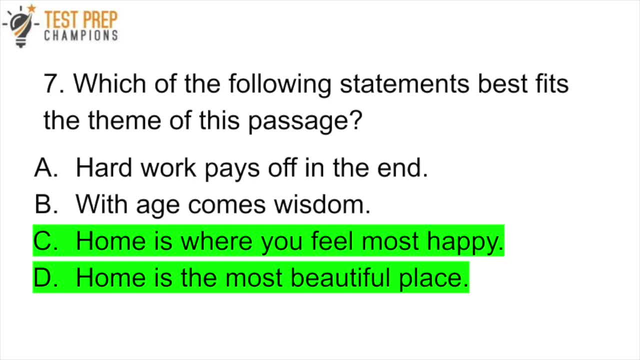 question that hits on multiple different things. so first of all, think back to question seven here. remember how i said that whenever you have multiple answers that are very similar in a multiple choice question, that one of them is probably the answer, and that this is especially true for answer choices that are mutually exclusive, or in other words, what i mean by. 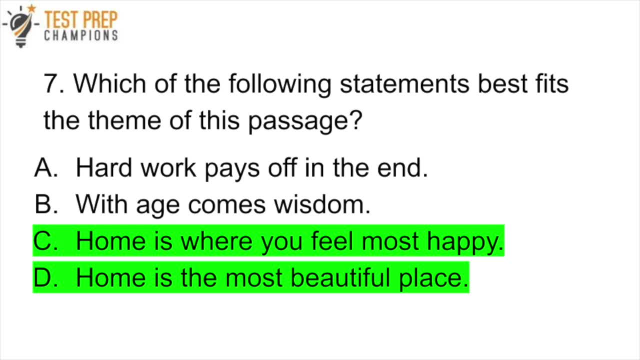 mutually exclusive is one question, when a question can have only one correct answer. so it would be impossible for both choices to be right. right if they are contradictory, or in other words, mutually exclusive. so since they both deal with home, right. so since c and d both deal with home as part of 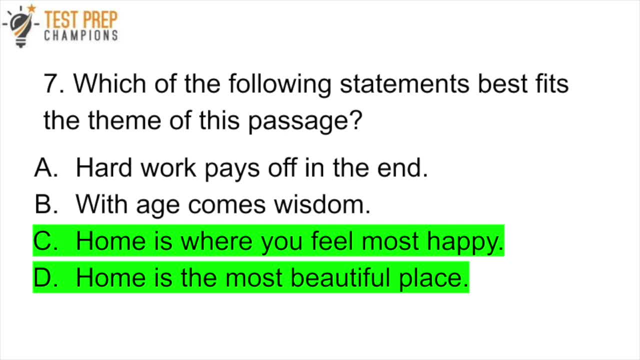 the theme, then remember we said that, logically, c or d one of them is probably going to be the right answer, and note that this trick isn't always going to work 100 of the time, but it's usually a good bet if you- especially if you- you're not sure what you have to do and you have to make a guess on the gd. 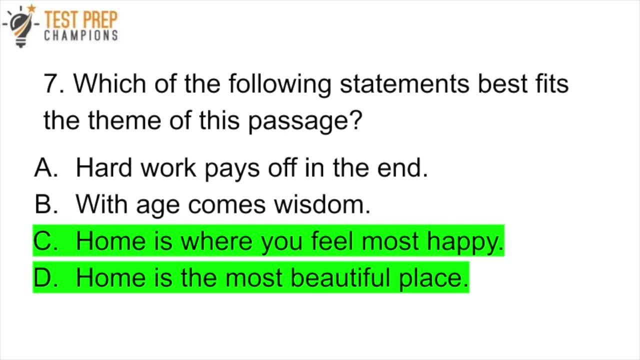 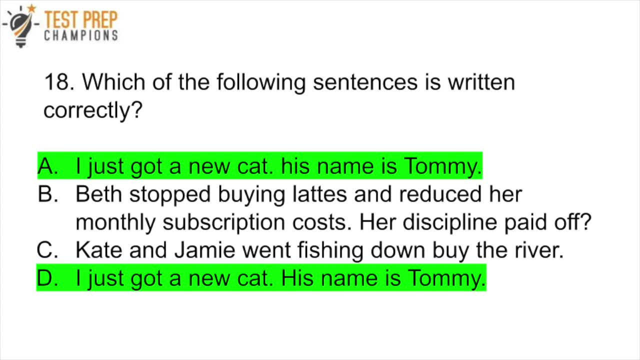 because on the gd you're always going to want to guess. you never want to leave something blank here. so we can use this trick to just narrow our focus down to a and d, okay, and so we see here that a and d are the same sentence, but there's two differences, right, and so we? we don't know for sure that it's. 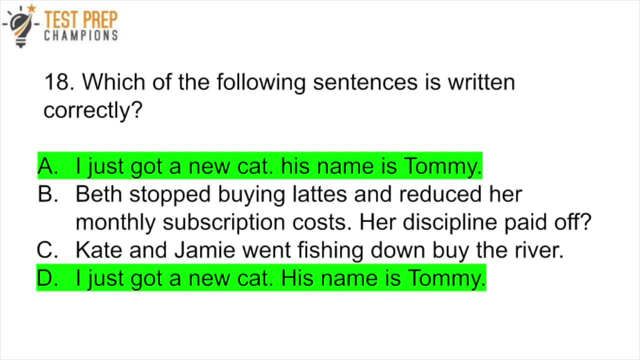 either a and d, but it's a safe bet, all right, that one of them is going to be correct, because and one of them is going to be incorrect, all right. so let's, let's break this down here, all right, and we're going to go over why each answer is going to be correct and one of them is going to. 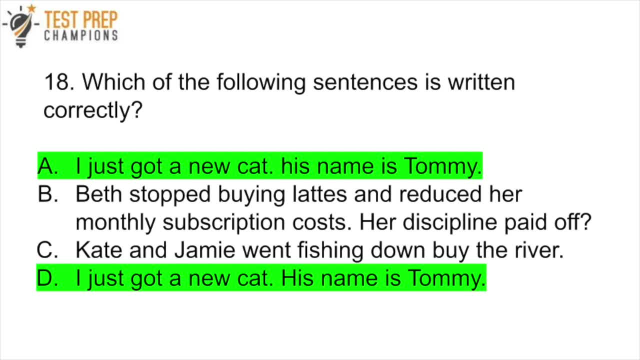 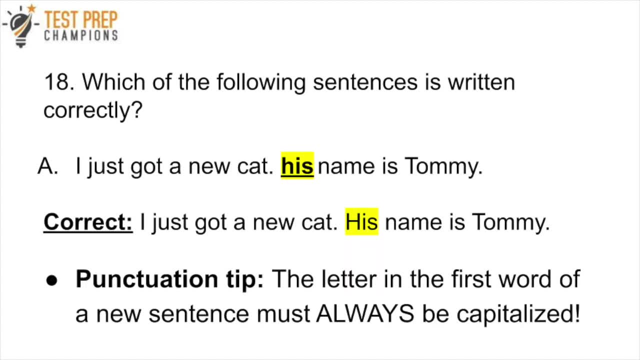 be wrong, all right. so a is incorrect and, as we know, d is the correct answer. so the key here is to understand punctuation. punctuation rules, all right, and so note that in your writing, you always want to start off each new sentence by capitalizing the first word in that sentence. so i've underlined and. 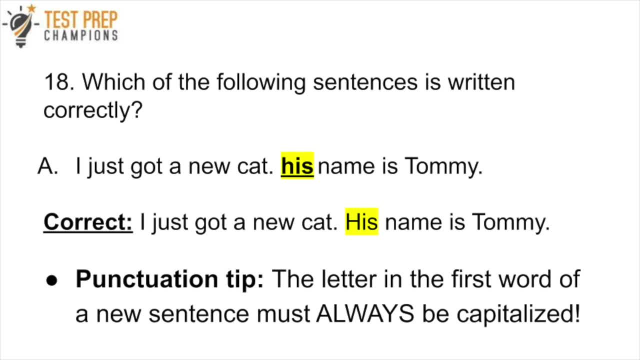 bolded and highlighted the word his in letter a because it's his with a lowercase h and that's incorrect. and again, the correct version is d. i just got a new cat, period capital h. his name is tommy, so the letter in the first sentence is correct and the letter in the second sentence is: 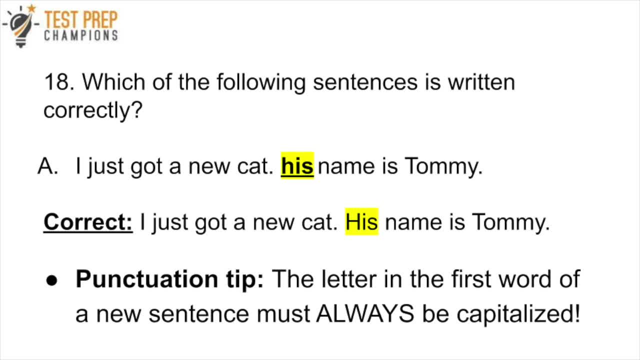 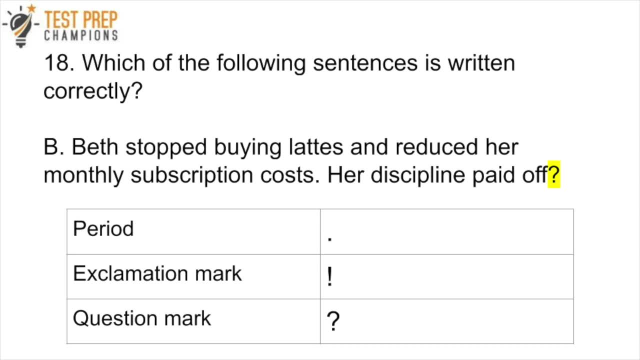 always supposed to be capitalized. okay, as a punctuation tip. now let's keep rolling here. what about b? why is b wrong? well, you need to understand that b is wrong because it ends in a question mark here. all right, and that's one of the reasons, but that's the one i want to focus on. 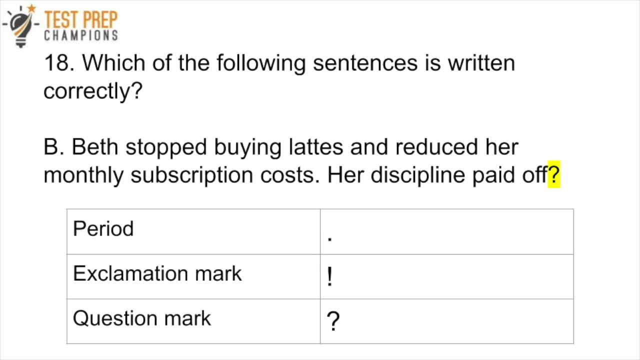 first here. so since we're we're on the topic of punctuation, all right, let's briefly review the three big types of punctuation. so a period ends a sentence and an exclamation. okay, so these are all three ways to end a sentence here, but the differences are that a period is used for a state. 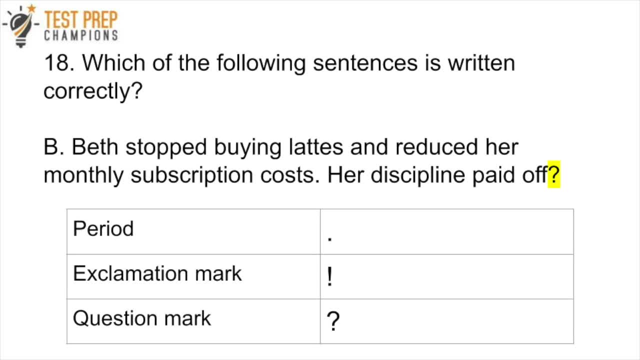 all right, and a question is used for a question, all right. now, an exclamation mark, which is also sometimes called an exclamation point, is for showing excitement or showing a strong feeling here. so in the sentence, her discipline paid off. all right, that's not a question. all right, we could. 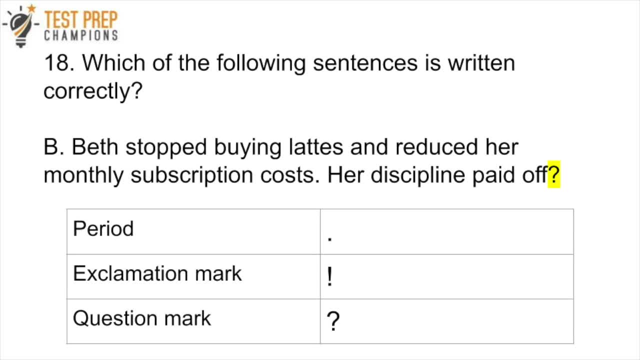 say, did her discipline pay off? or or, in the long run, did her discipline pay off, something like that, but her discipline paid off. okay, that is supposed to be a period at the end. so that is why a b is incorrect in 18. now, as a general rule of thumb in your writing when you're writing a sentence. 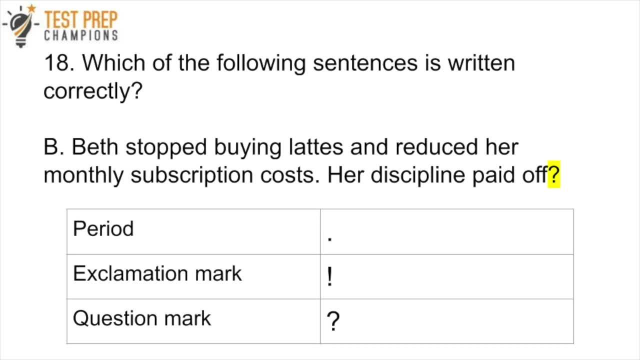 writing. i recommend sticking mostly to periods, just to be safe, because you know if you put an exclamation mark or a question mark somewhere where it's incorrect you might lose a point for that. so i would stick mostly to periods. there's not much of a reason to use exclamation marks or 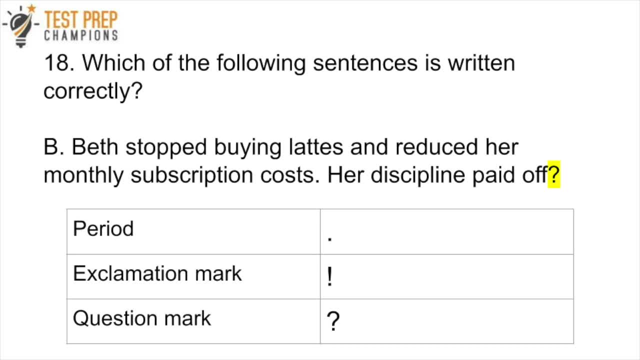 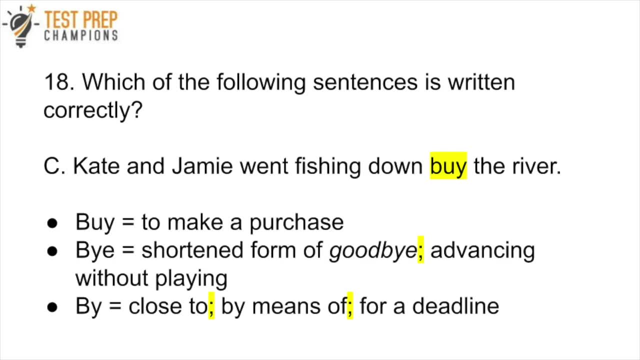 question marks. now, if you're confident that you're using them correctly and you want to throw a couple in, sure why not. but i i generally recommend avoiding it. there's usually no need to do it, okay? so what about c? what's wrong with c? so c is wrong because the word by is not the correct form, so 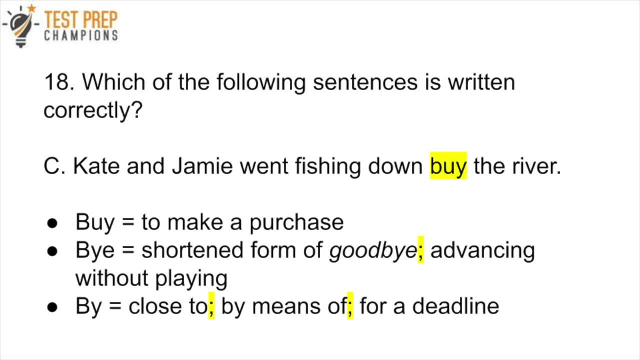 again. this is another example of a period in a sentence where a, b is incorrect and a question of words that sound the same but are spelled differently and therefore these words have different meanings. so we've got by spelled b u y, which would be to make a purchase, like i went to. 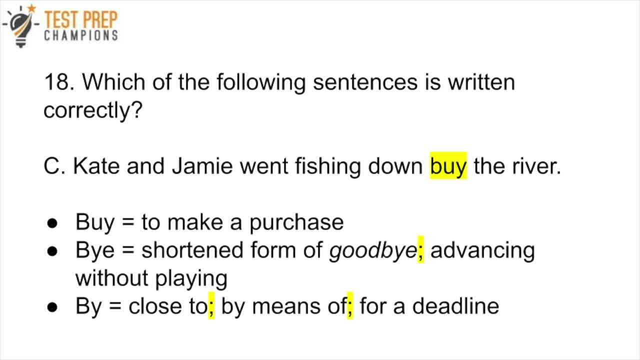 the store because i had to buy something all right now. the word by b y e can mean two things. it could be a shortened form of the word goodbye, like he said bye. or it could be like: think of a sports team. they had a bye week. all right, a bye week would mean that the team advances to the next week. 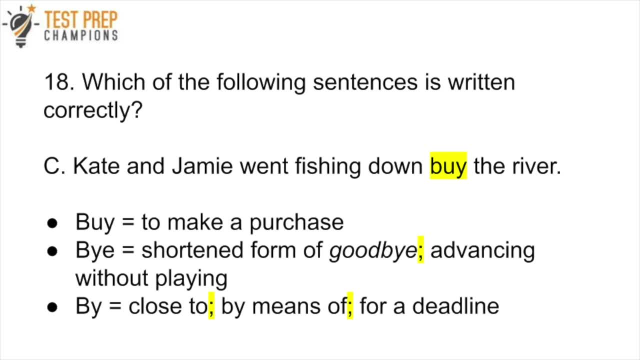 without playing, or if you have a buy in a tournament and then you skip that first round of that tournament, you go right away to the next round. now, by spelled b, y would have us as a couple different meanings, but the ones that are most important are meaning close to, which we see here. okay, they went fishing close to the river, that's. 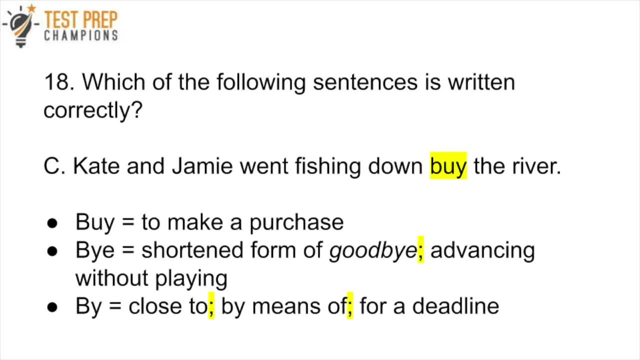 what we mean by by in the sentence here. also, by could mean by means of, like, for example: um, he passed the ged test by studying every night of the week for a couple weeks in a row, all right. and it also could mean for a deadline, like he had to take the ged test by january 1st, all right. so 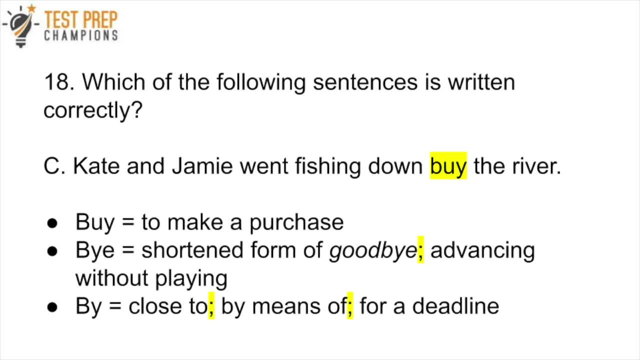 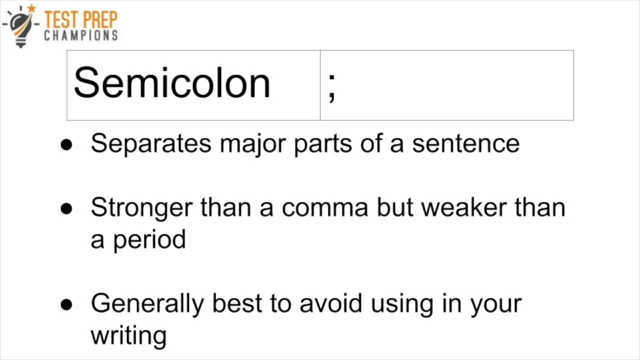 those are just some examples here. now i've also highlighted the semicolon. so you might notice the semicolon things, that what they look like is just a period on top of a comma and the best way to think about them is that they are stronger than a comma but weaker than a period. all right, that's. 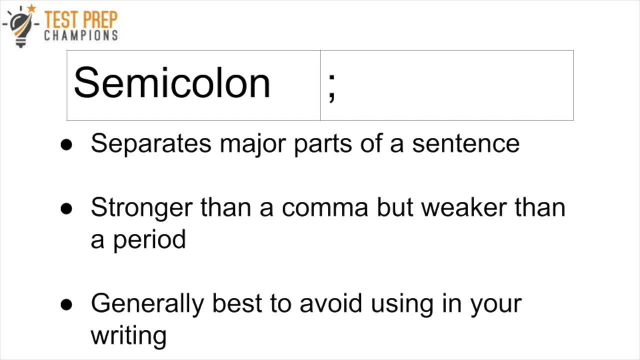 just kind of a a way. i don't know if it's the grammatically correct way to say it or not, but that's a good way to think about it. all right, and semicolons can be used to separate parts of a sentence. all right, and the most common use of a semicolon is to join two independent clauses. 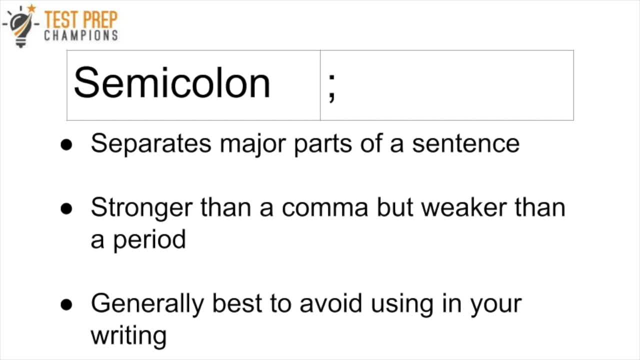 without using a conjunction, like a word such as and or but. so conjunctions are words like and or but and they they're going to follow a comma. typically all right, although sometimes people don't write a comma after the conjunctions, but in most cases you would technically want to do that to be. 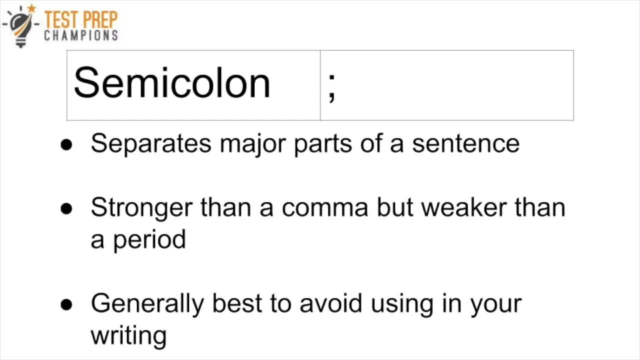 grammatically correct. um, now, what about the word clause? what do i mean by independent clause? well, an independent clause is just a way of saying a complete sentence or a sentence right. a dependent clause? there's a group of words that contains a subject and a verb, but it's not a complete thought. 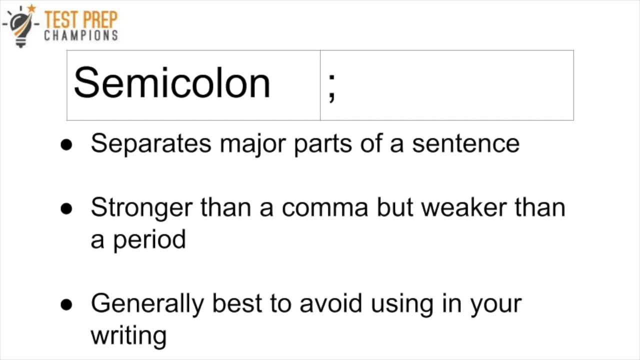 unlike an independent clause. all right, and so again, just like with exclamation marks and question: all right, so these are generally- uh, there's no use to use them in your writing for the essay. now, in real life, of course, there's plenty of purposes for using them, um, and you're going to see them in. 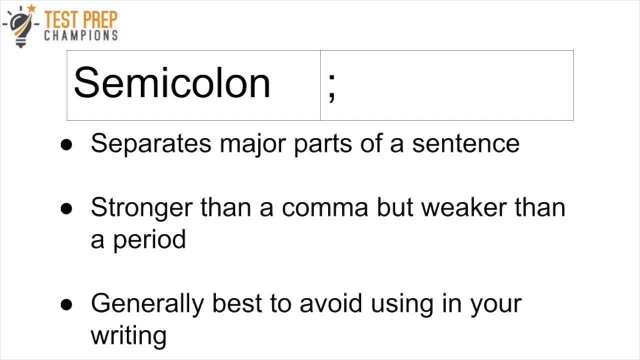 your reading, so i wanted to make sure that i addressed what that was. but just know that in your own writing, for the purposes of the essay, i just recommend not using them. okay, just end the sentence with a period and just start a new sentence. capitalize the first letter, that first. 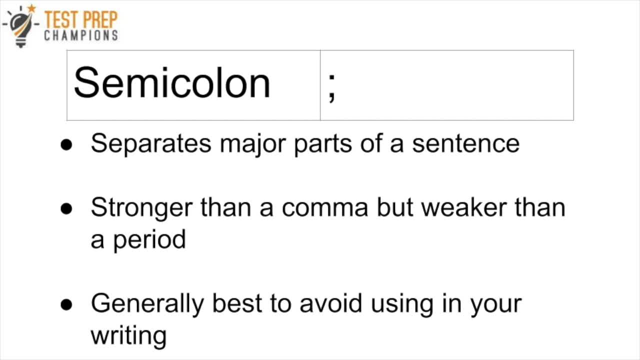 word and just go on with a new sentence, just because it's kind of like you know there's. if you're not a hundred percent sure that you're using a semicolon in the right place, just don't even take that chance. all right now. of course, if you feel comfortable with them, go ahead, but that's. 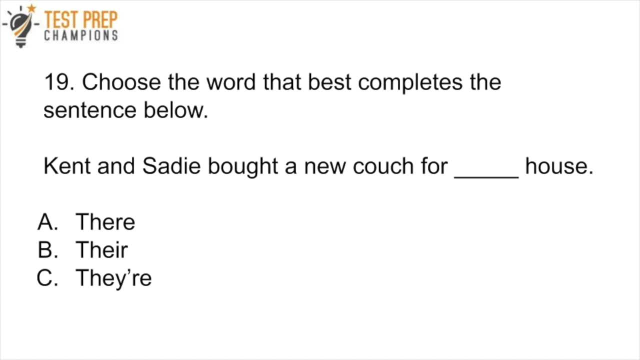 a choice you have to make, so let's move on here. uh, to number 19. now, all right. so in number 19, choose the word that best completes the sentence below. so kent and sadie bought a new couch for blank house. choose the correct form of their a, b or c. pause the video and go ahead and give that. 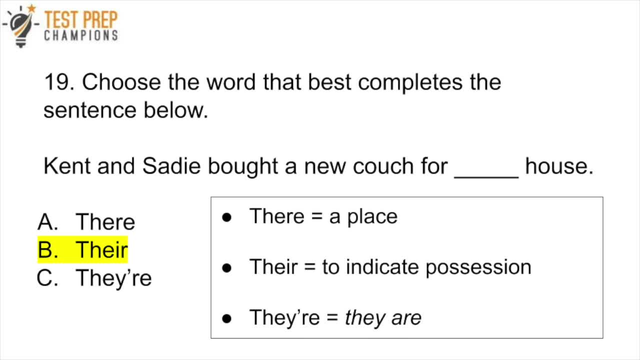 a whirl right now, okay, so let's go over this. so, basically, what you need to know is, first of all, b is the right answer, t-h-e-i-r is right and these are. there is another common word, that it's. there's three different ways to write it and they sound essentially the. 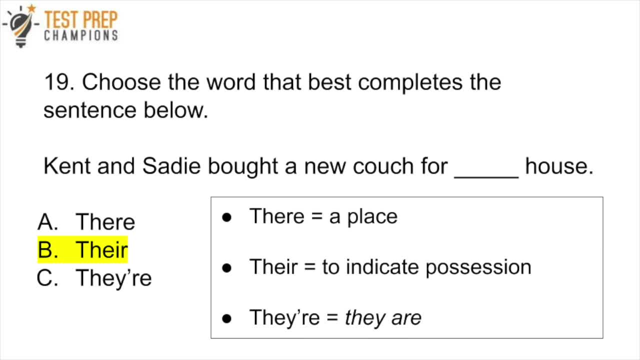 same but they're spelled different. all right, except c there, okay, b there, a there, right, they all sound. they all sound the same, but they are spelled differently and they mean different things. so there, t-h-e-r-e would be used to talk about a place like they are going over there. all right. 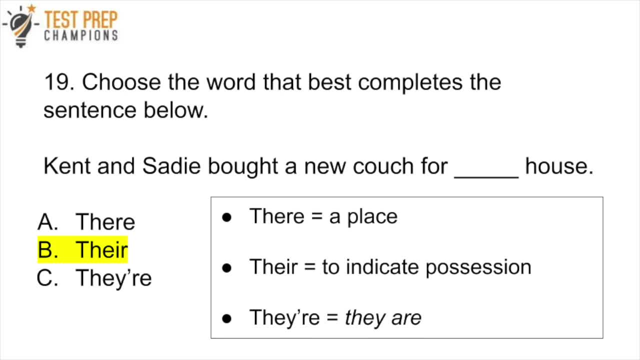 over there in the city. this happened all right, for example, and you can remember that by the word here h-e-r-e, so you would say i'm here like a place we'll think of there. it's having that word in it all right, and they're spelled t-h-e-i-r is to indicate possession and that's why this is the. 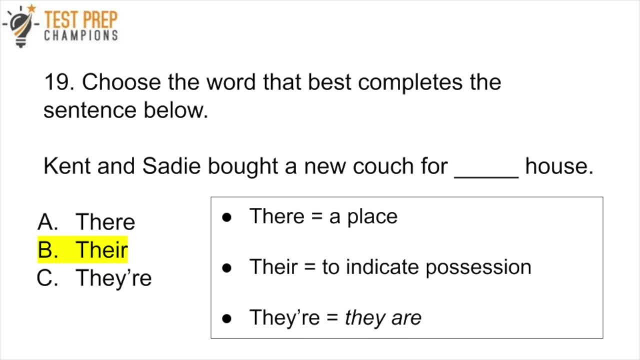 correct answer. so ken and sadie bought a couch for their house. they own the house, all right, this is my book. or you could say that's their book, that's their ball, that's their pet, whatever, if it's talking about possession, it would be t-h-e-i-r and they're spelled t-h-y, apostrophe, r-e. that's just. 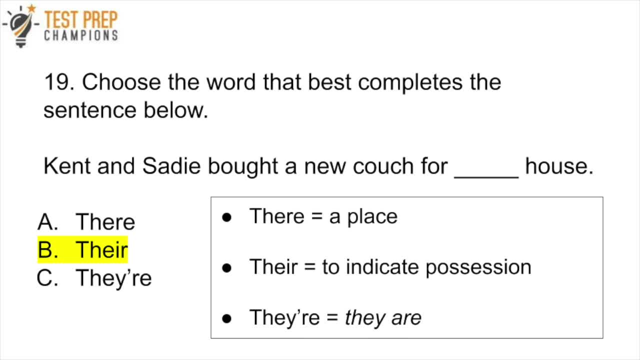 means that it's replacing they are, so two separate words. they are there with t-h-e-y apostrophe r-e is replacing they are. so you could say maybe, uh, kent and sadie went to the school. they are there now. all right, meaning they are there now, but you, instead of saying they are as two words, you. 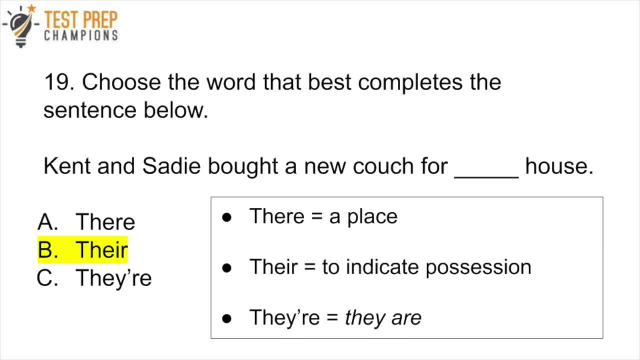 would just use. they are uh, with the apostrophe, they apostrophe r-e. all right, so this is really important to know. um in for the test in general, but also for your essay. all right, um. so now let's keep moving here. 20, which sentence is written correctly? go ahead and pause the video and take. 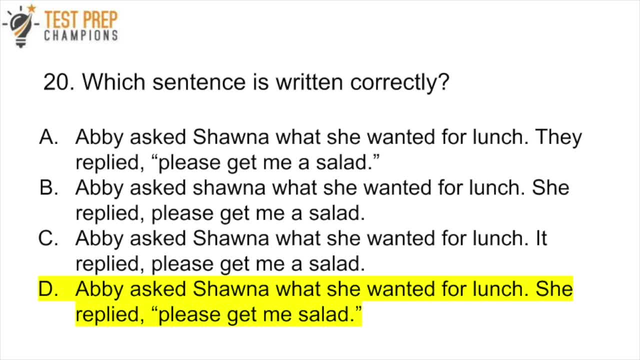 a stab at this one, then, of course, we'll go over it. d is the correct answer, but we can't just stop there. let's break down a, b, c. and why is d is correct? because this is has some very, very important lessons for the gd test. so let's 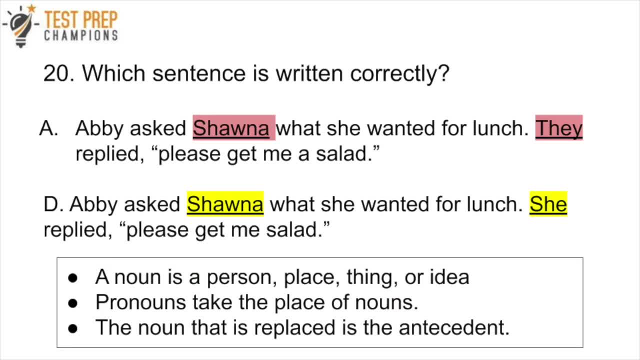 compare a and d. so basically the sentences sound exactly the same, but the main difference is the word they versus the word she. okay, and we have to understand first of all what a noun is. a noun is a person, place, thing or idea. and we also have to understand what a pronoun is. a pronoun takes the 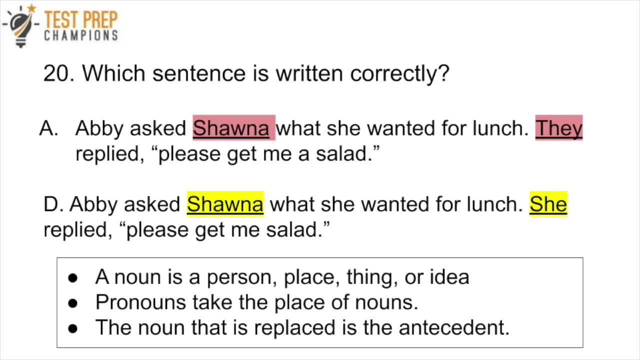 place of a noun, all right. so pronouns are substitute nouns. they substitute for a noun or nouns, and so whenever a pronoun replaces a noun, know that we call the noun that was replaced the antecedent. okay, the noun that gets replaced by the pronoun is what we call the antecedent. so here, 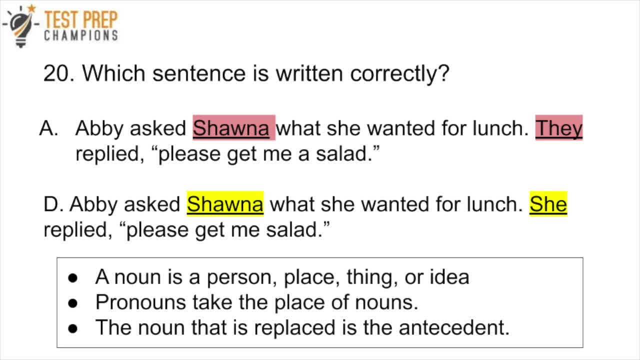 shauna is the noun and she is the antecedent. so noun and pronoun agreement is very important for your test. the noun and pronoun must agree, in other words. so since shauna is just one person, we want to say she instead of they. if it had been multiple people, we would say they, but for one. 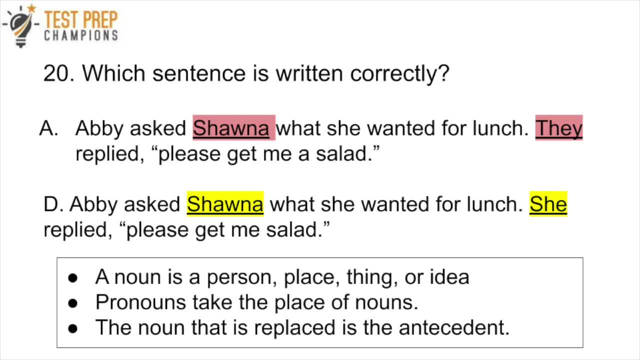 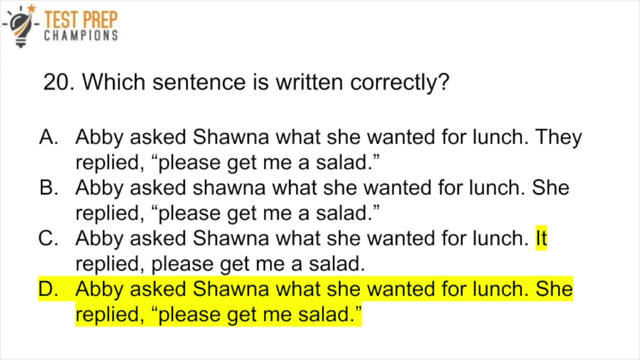 person. we say she, so therefore d is correct. so now that we see why a is wrong, we can see that c is wrong for a very similar reason, but it's a little bit different. so the word it is what tells us that c is wrong. so, and also the fact that there 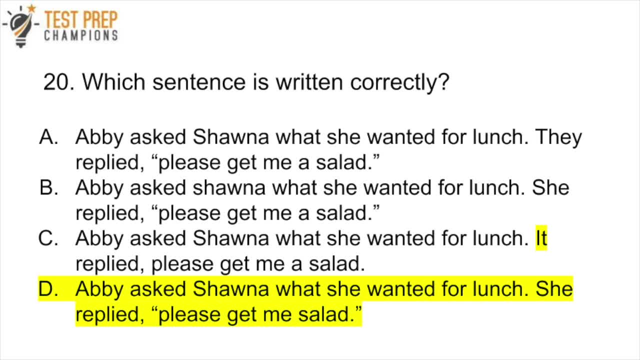 are not quotes around. please get me a salad. but the main thing here to understand, besides those quotations, is that it is usually used to take the place of an object or a thing, not a person. all right, so that's why that is incorrect. so we now know why a is wrong and we know. 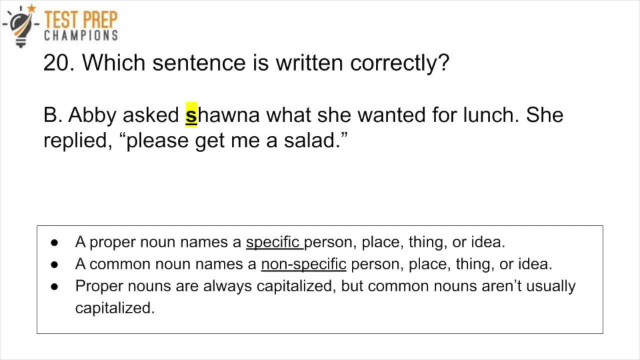 why c is wrong. but what about b? b is the last one standing here, so let's go over it. so in b, what we have to understand is the difference between proper and common nouns. okay, and so a proper noun names a specific person, place, thing or idea, whereas a common noun names a non-specific person place. 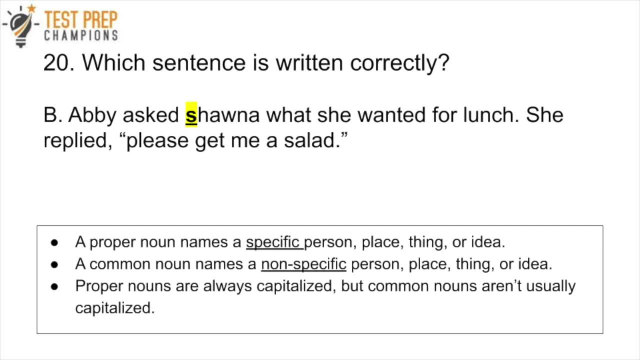 thing or idea. now, proper nouns are always capitalized, but common nouns usually aren't capitalized. so you can usually tell proper and common nouns apart, because with proper nouns the first letter is going to be capitalized, like i said. all right, this is almost always the case. however, with a 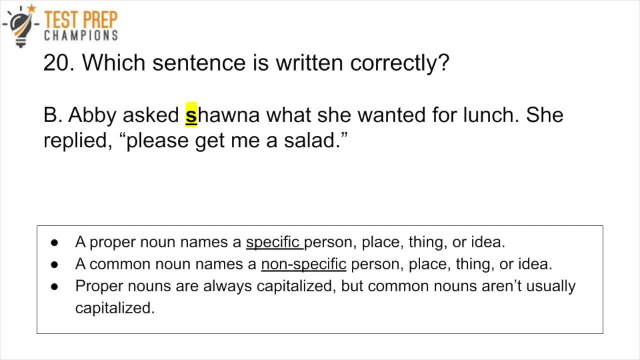 an improper noun or, like i said, a common noun. all right, it's almost never going to be capitalized. the only exception that you would have to understand for the test is that if a common noun is the first word in a sentence or if the common noun is part of, like a book title or 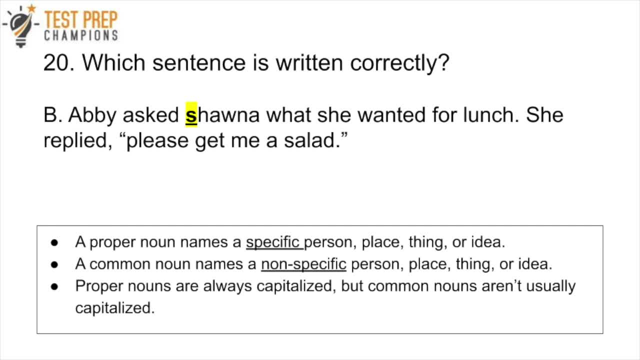 something of that nature, then it might be capitalized, but for any other reason, all right, the it's not going to be capitalized, all right. so that's a good way to tell them apart. and really the difference is that a proper noun would name like a person, like you would say: uh, barbara went.